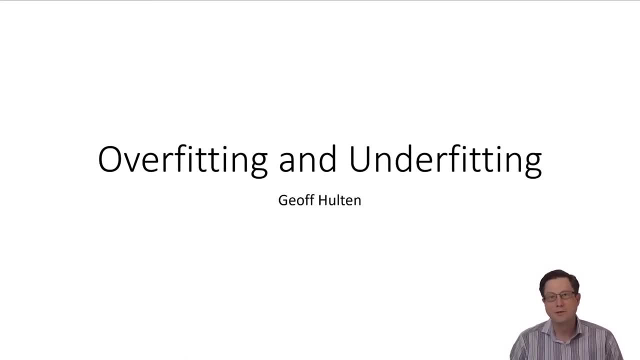 All right, everybody, good to see you. There is just some major thunder and lightning, unbelievable, but I think we'll survive. And now we're going to talk about overfitting and underfitting. I think we're going to survive that too. Anyway, overfitting and underfitting. 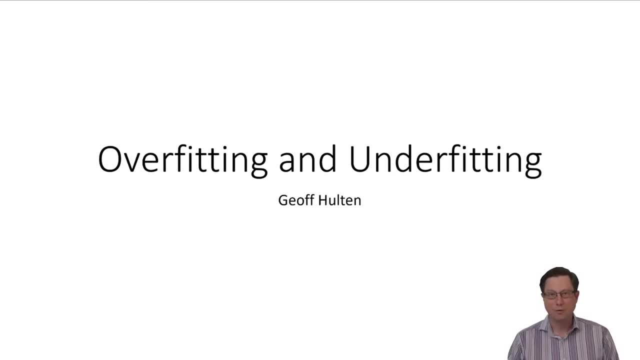 is one of the primary challenges for why machine learning is hard is: how do you balance the ability to learn the concept you're trying to learn without getting confused and lost and gibberish and noise. So we're going to go through this concept today. look at it in a 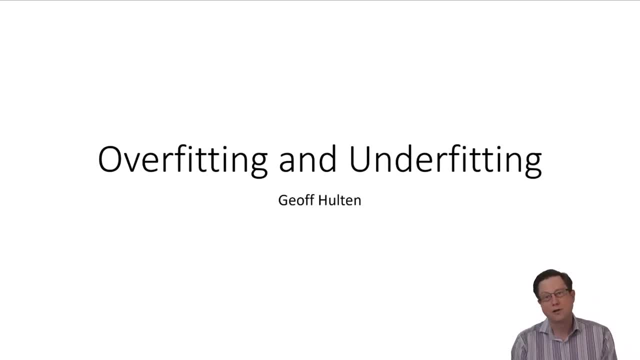 couple of different ways and hopefully get you to the point where you can start including thoughts about controlling overfitting and underfitting in your model building process as you're setting up the hyperparameters in your model search process. So there you go, Let's start. 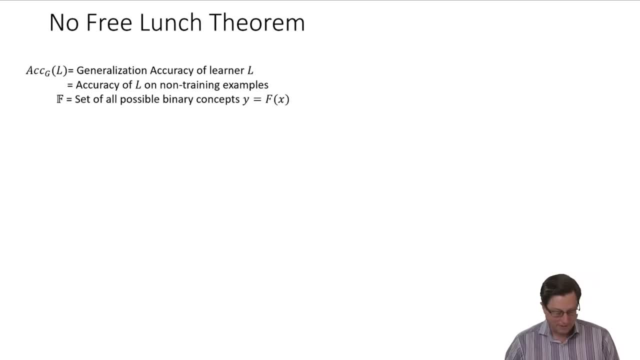 with a little theorem, a little bit of math, but it's really just for a concept. The theorem is called the no free lunch theorem And what it says is that if accuracy sub g is the generalization accuracy of your model, then you're going to be able to control overfitting and underfitting. 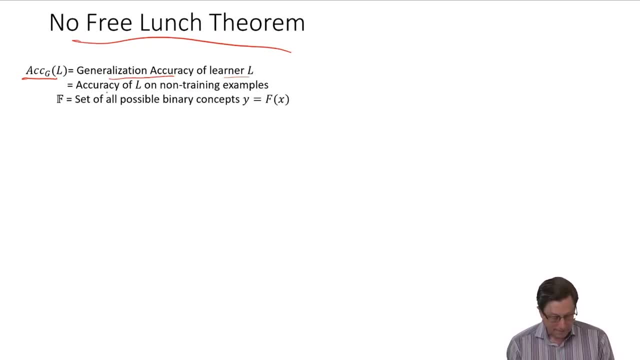 your learner L, That's the accuracy of the learner on non-training samples. so on your test samples or actually on the performance time samples And for the rest of this slide I call that sort of like the generalization accuracy or generalization samples as the 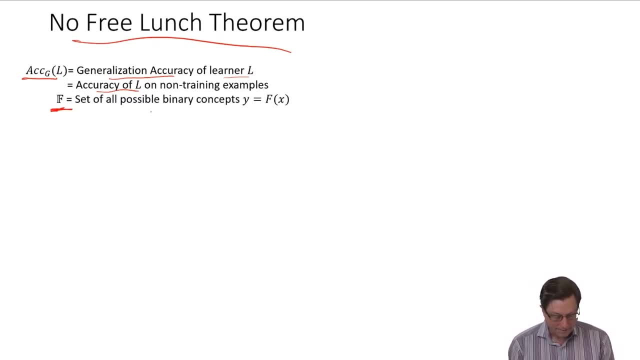 non-training samples. And F is the set of all possible binary concepts. I don't think binary is important, but there's every possible y equals f of x that you can think of. that's possible in the world that you're working in. Then there's this theorem, the no free lunch theorem. And what? 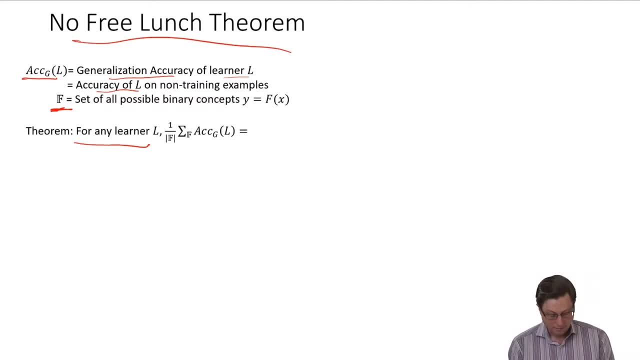 it says is that for any learner that you have, and what this says is: this is the average generalization accuracy over every possible concept. And what do you think? it is The average generalization accuracy over every possible concept? And here's a setup. You have your. 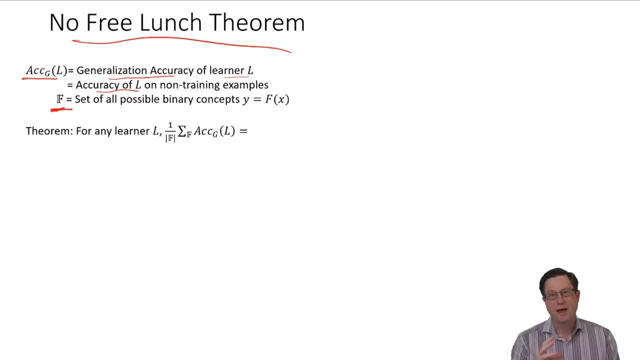 training data and you build a model on the training data you have and then you deploy it. The training data, presumably, was drawn from the concept you're trying to predict on, But we all know that. you know there's statistics, there's everything is an IID sample, So there's a 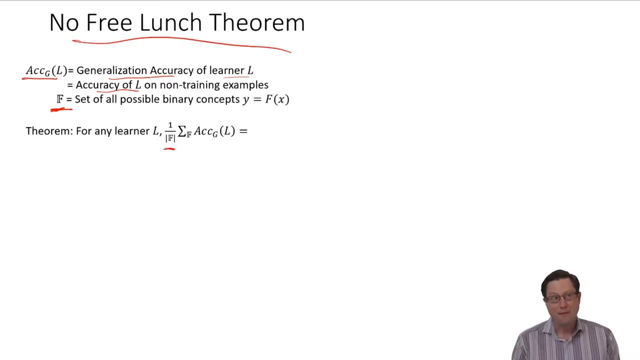 probability that the training data you have is not a good representation of the concept you're trying to learn. So you know, in a mathematical sense, you know with this, like we want to prove a bound and we want to say, well, what is the average accuracy, generalization accuracy of any 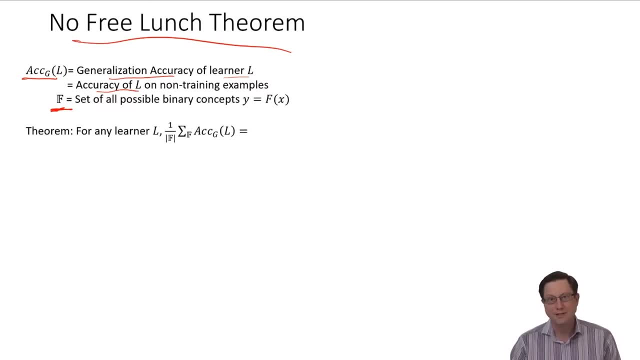 learning algorithm, Like why are we doing this machine learning stuff So we can generalize, must be pretty good, Turns out, average generalization algorithm accuracy of any learning algorithm is 50%- 50%. What are you talking about? Remember, this is a mathematical bound, It's not exactly a. 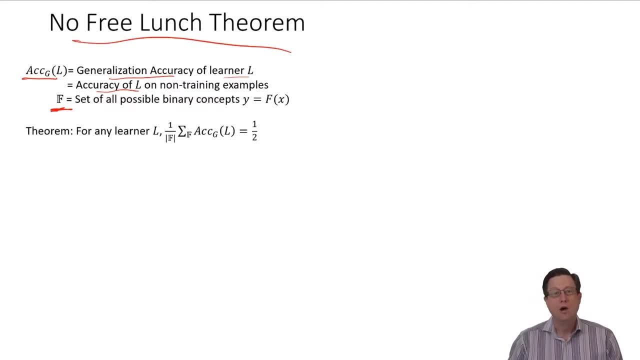 practical thing, But it's a good way to start thinking about this overfitting and underfitting concept, which we are going to talk about more in this lecture. So let's think about this a little more. It's a little crazy. So let's now we have two learners, learner A and learner B, And we're 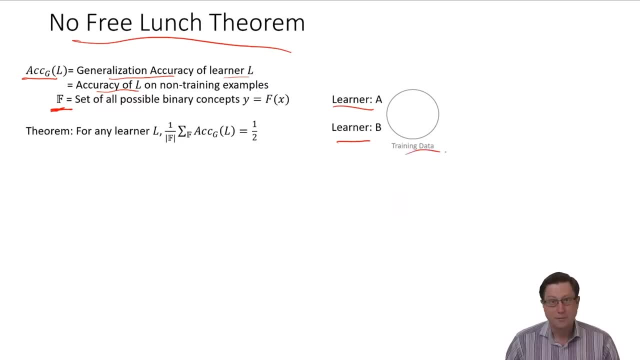 going to try to build a model on So fine They both build a model- And on the training data, one of them has great accuracy, One you might as well be guessing. Learner B did not do a good job at this. 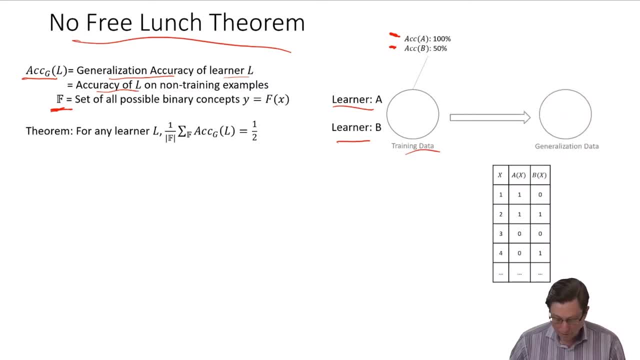 concept. It doesn't matter. That's on the training data. What we want to talk about is the generalization accuracy of these models that we've learned. Now we can go through and do all the statistical bounds, But again, this is more of a theoretical machine learning theory result that 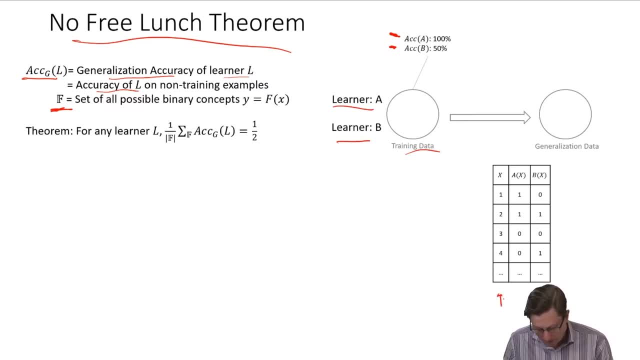 we're talking about here. So if you're interested in learning more about this, you can go to the link in the description below. So if you say, here's the samples- X1, X2,, X3, X4. And here's what, the prediction of learner. 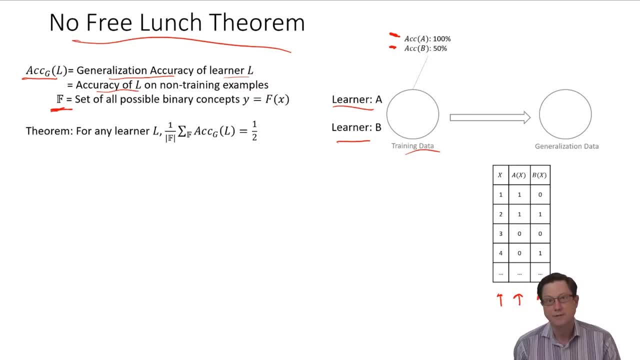 A's model and learner's B model is on each of those samples. Now, when you're talking about the set of all possible concepts, what a concept is is that it can take any X and map it to any Y. That is what the concept is, And in machine learning we're trying to recover that concept. 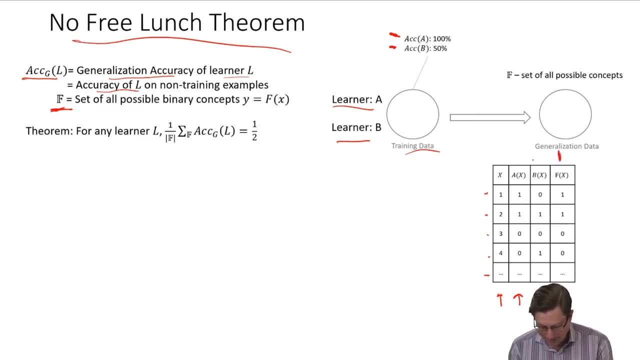 But you could have a particular concept that takes X1 and maps it to 1, X2 and maps it to 1, X3 and maps it to 0, X4 and maps it to 0. You could do that, no matter. 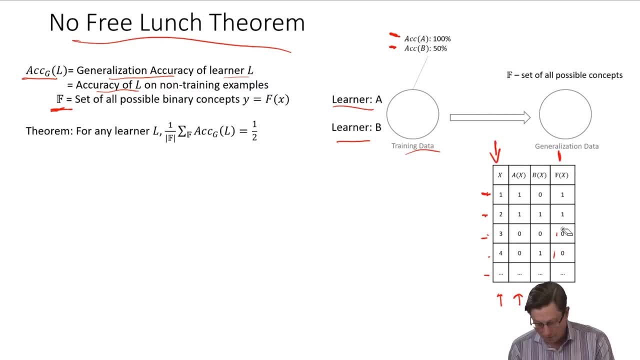 how many features X has, what those feature values are. The underlying concept could be that It could be. Why not? In that case, you can see that your generalization accuracy would match your training set accuracy And you'd be like, haha, that's great, And we can use statistics. 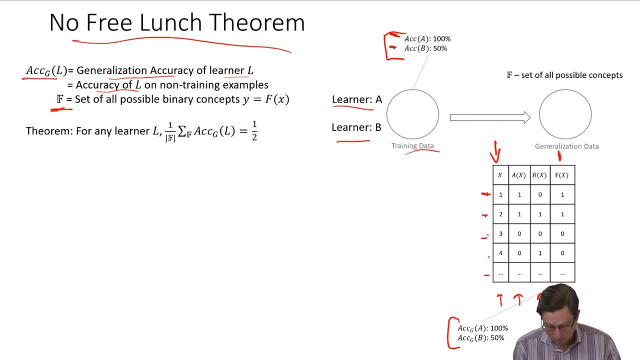 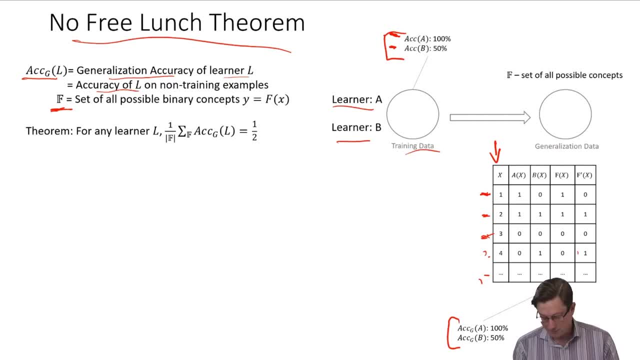 I mean that exists, You could write it down. It's just a different combination of the features that happen to be in X. The process uses those and creates something different. Remember, this is all like kind of in terms of the raw stuff and your feature engineering is going to happen and 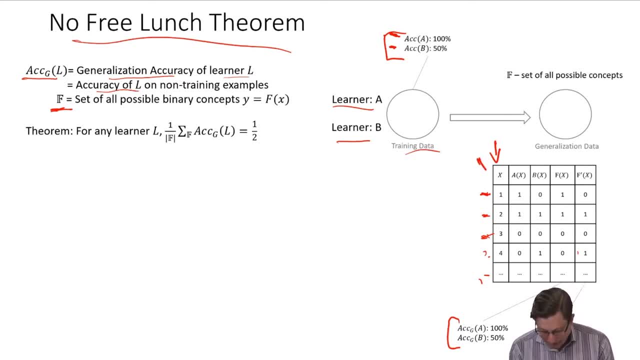 et cetera, et cetera. But in this case the generalization accuracy for that set of features concept for learner A is 50%- Okay, For learner A is 50%- And the generalization accuracy for learner B is 100%. It's exactly opposite what we saw there, exactly opposite what we got on our 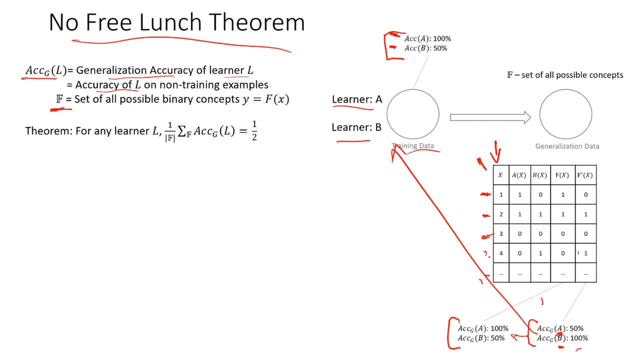 training data. It's unlikely statistically that this would happen, but it's possible. There is such a concept that could cause this to happen if you want to get pathological, And so that's kind of like the sense of there's no free lunch. 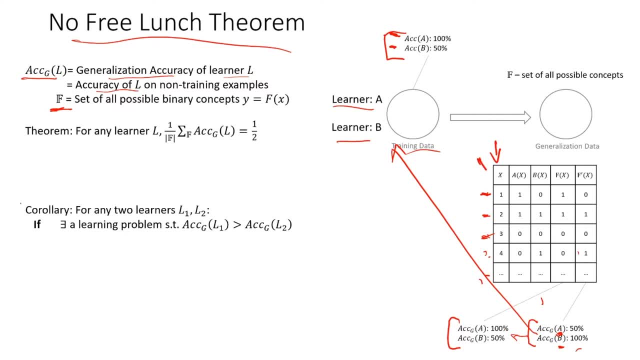 And when this corollary will drive it home a little bit more For any two learners, L1 and L2,. if there exists a learning problem where learner 1 gets a higher generalization accuracy than learner 2 does, then there also exists a learning problem where learner 1 has a lower generalization. 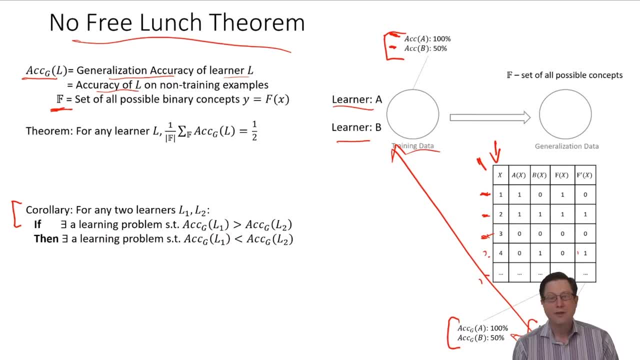 accuracy than learner 2.. And you could think of it just as like, sort of in an adversarial sense, where you pick the training data that you apply learner 1 to and learner 2 to, and you pick the training data in such a way that learner 1 will get you know, let's say, 60% accuracy on your. 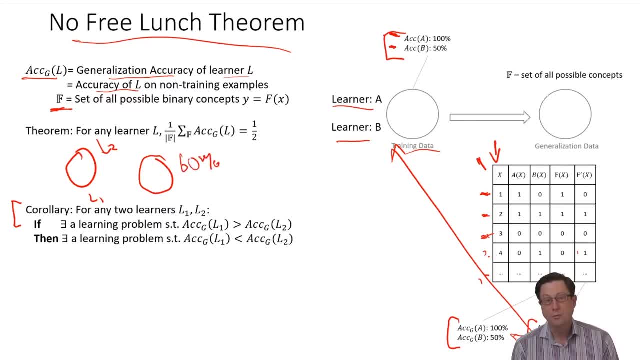 holdout test data, Right. So then learner 1 would be better than learner 2.. Now you just flip all the labels on the test data. Now just the opposite algorithm has the 60% accuracy and the other one looks worse. So that's a little bit more complicated. But it's a little bit more complicated, So that's a. 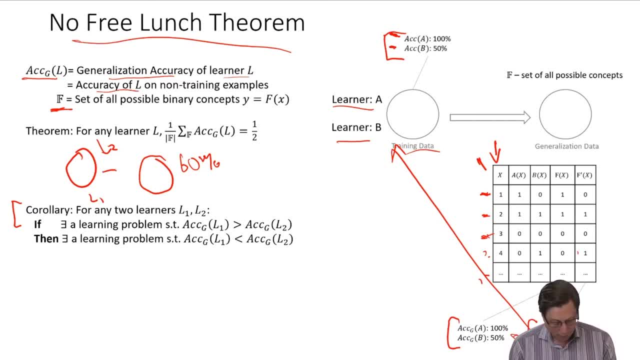 little bit more complicated, But it's a little bit more complicated, But it's a little bit more complicated. So in some sense you know, anytime there is any way that learner 1 and learner 2 differentiate what's going on in the concept and have some different opinion about a part of the 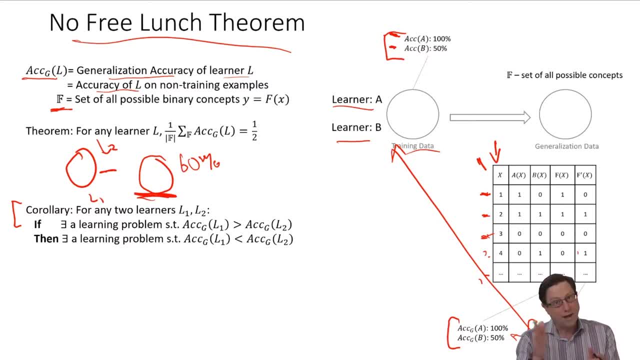 concept. then the concept could be the way learner 1 learned it, or it could be the way learner 2 learned it, and either could happen theoretically. And so the way to take this home and what you should think about- and you know this is a little bit of like a theory thing and there's kind of 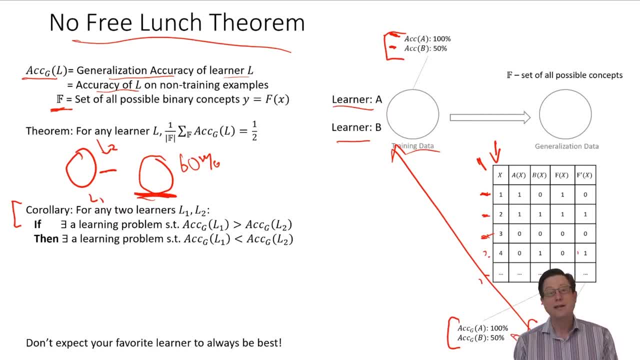 a trick there and it's not very practical. But the underlying point is quite valid, And that is: don't expect your favorite learning algorithm to always be the best, Because no matter how well you know how to use it, how much data you have, how much more. 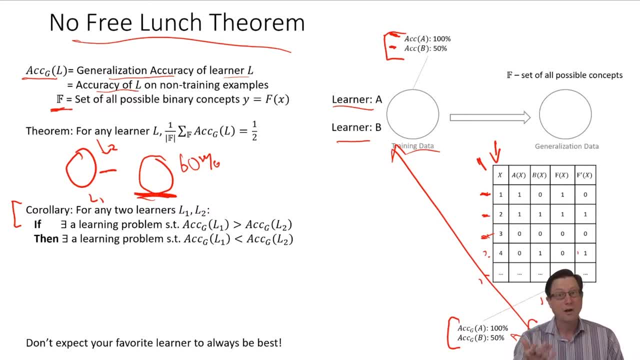 powerful, it seems, than another learning algorithm. there is a concept where your favorite learning algorithm doesn't do as well as you know a simpler learning algorithm or somebody else's favorite learning algorithm or something along those lines, And, that said, you know like. 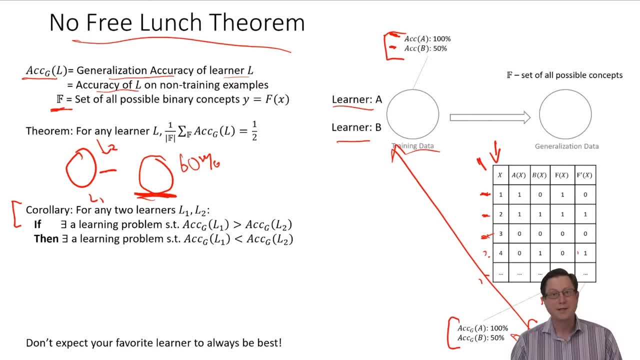 I talk about the toolkit, logistic regression, boosted trees and neural networks as a great set of things to learn and to use, But they're not always going to be best. not for any problem that you might bump into, just for many, many problems that you might. 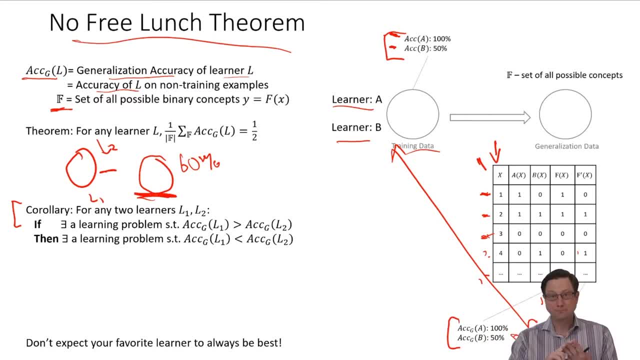 bump into in practice. And in fact, I didn't just say one, I said three, Because each of them is appropriate for different settings with different constraints. Okay, so no free lunch. the one you like the most won't always be the best. That's what you got to think of. Okay, and so why is it? 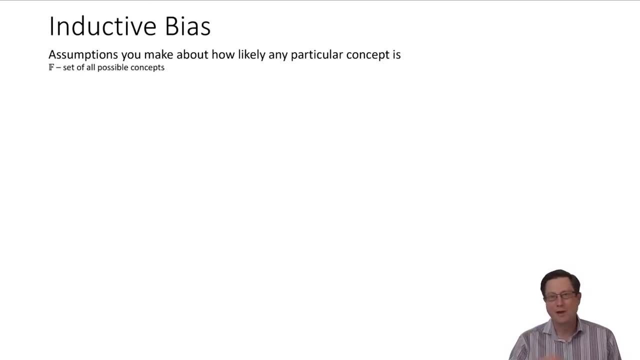 that one particular learning algorithm or learning setup, training or training approach is not always best And you know, certain concepts will be good on, certain concepts it won't be good on. And to think about this, you need to understand this concept of. 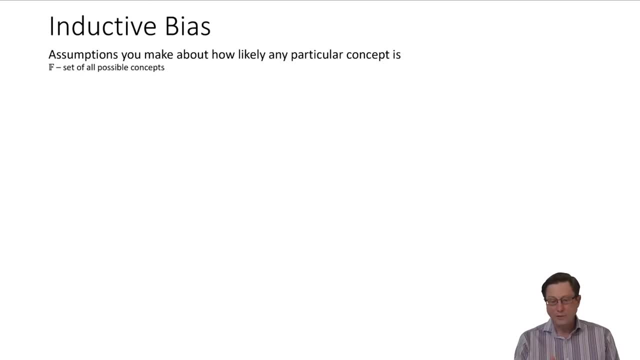 inductive bias. Now, inductive bias is when you set up your learning process. just by how you do feature engineering, just by which hyper parameters you try, just by what model structure you choose to use, you encode assumptions about how likely any particular concept is. So once you've decided, 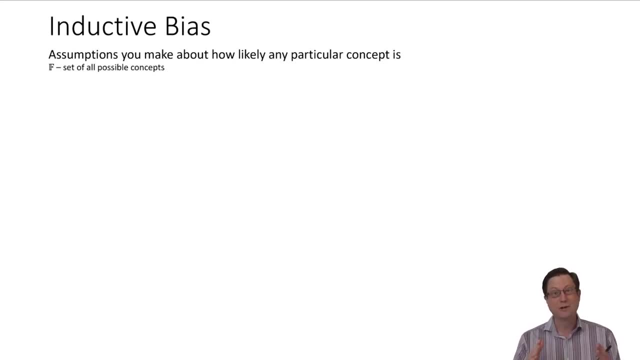 you're going to use a linear model, that nonlinear concepts are extremely unlikely because you can't learn them right. They just don't exist anymore. Once you've chosen to use a decision tree, you've encoded a different set of assumptions and that becomes your. 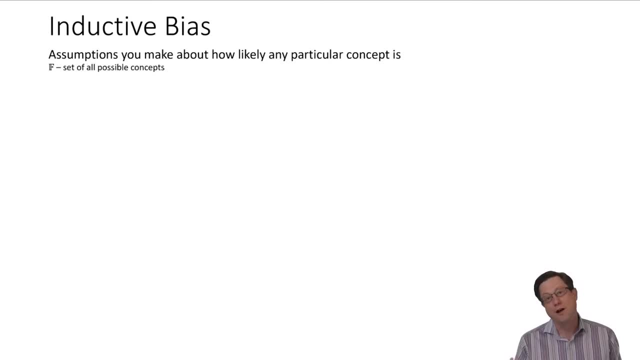 inductive bias and then that tells you what types of concepts you are better on and what types of concepts a different algorithm might be better on. So common assumptions are like I just said. the model structure: Is it a linear model? axis-aligned tree structure? Do you want to have decision trees that can split? not. 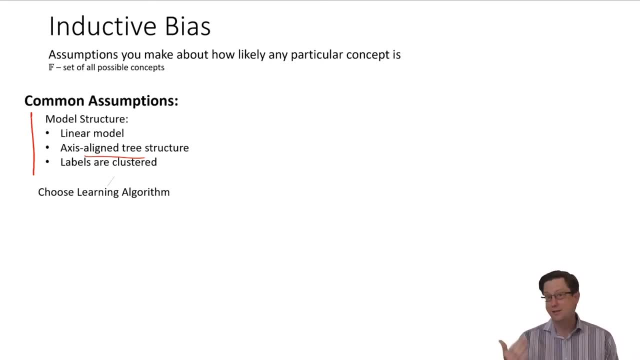 axis-aligned. You could do that. I don't know That would be a different inductive bias. You'd need a different learning algorithm, but it's certainly doable. And another thing is that the labels of one, you know all the y equal 1 labels are: 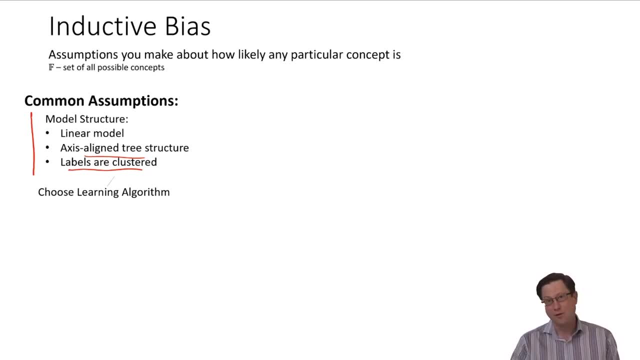 kind of near other y equal 1 labels and all the y equals 0 labels are kind of near all the other y equals 0 labels. and you're not in this pathological world where every other, like nanometer of instance, space, changes class, label And so 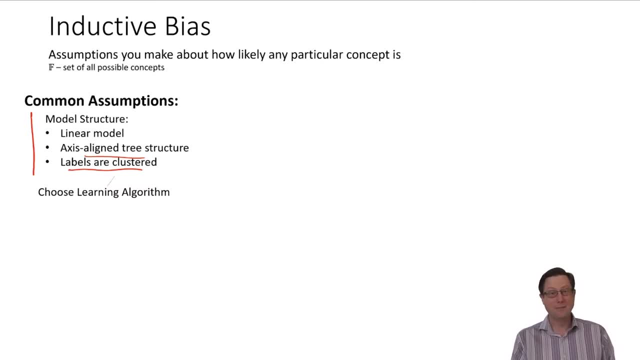 that's sort of what I'm trying to do here. I'm trying to figure out what the most common thing for inductive bias is, And I guess what we can do is, you know, every message that is a spam looks kind of like other spam messages, It's not? 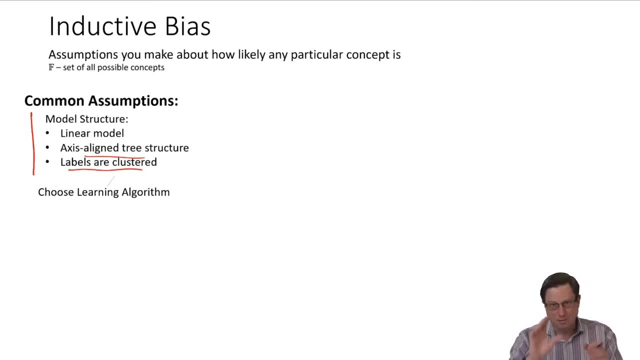 like it looks almost like exactly like a good one, and blah, blah, blah, blah, blah. And there are other types of inductive bias you have, and here we talk about even just the process that we use to do our training, The fact that we take our 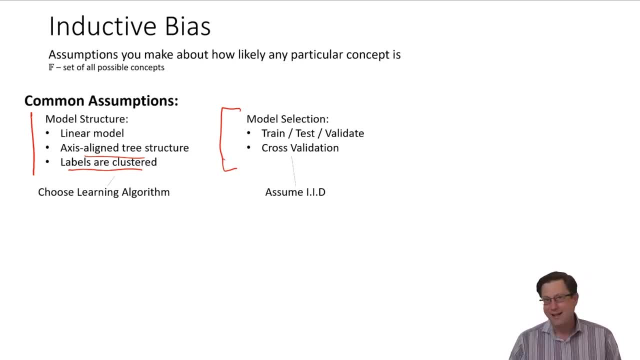 available data and split it up to train, test and validate, and we use the validate data to tune hyperparameters. but even more than that, we've used the our intuition about setting up well which hyperparameters are. are we even going to try? Because you know, like I've said many times, machine learning is the art. 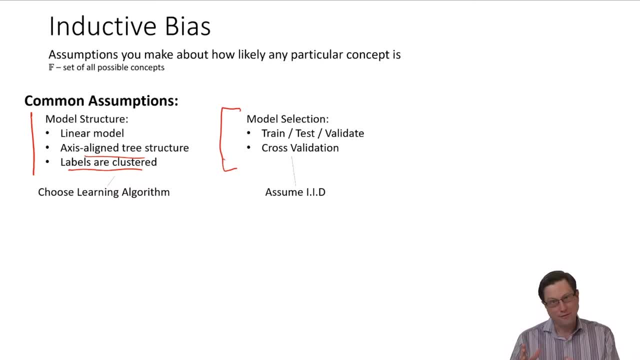 of you can't try everything, And so another way to think of your inductive bias is: well, which things do you just not try? And why do you choose not to try them? Because they typically don't work. You have experience. Somebody who's done a lot more machine learning than you gives you. 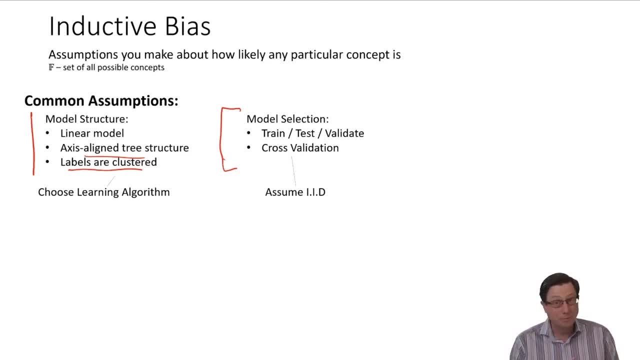 you know here's a good range of where to look at that hyperparameter, But there's plenty of other things you could try. And if you try those other things, I you know theoretically there's a concept that you would do better learning that concept by using a crazy value of a hyperparameter. 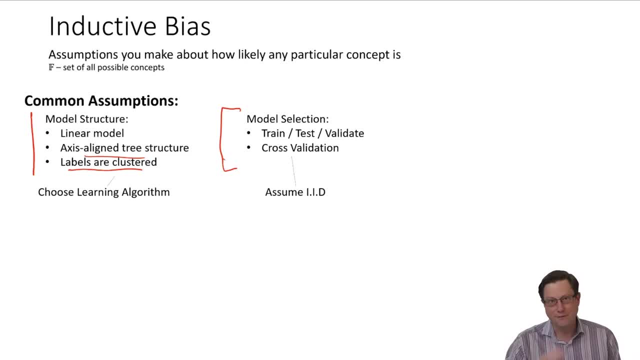 than by using the hyperparameter that everybody would always use or the value range that everyone would always use. Even this assumption of IID is an inductive bias And, as we've seen with time changing concepts, it's one that is very commonly broken in practice. And then you know we have 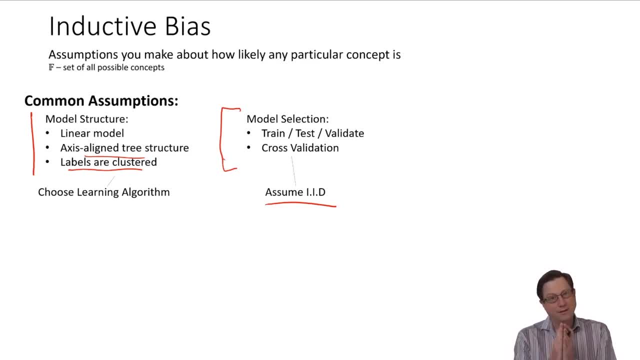 this bias of: oh, let's train, look at the data as a time stream and cut back like a few days and use the data before that to train and the data after that to train, And then you know we have to set thresholds. All of that is forms of inductive bias that you're bringing to the. 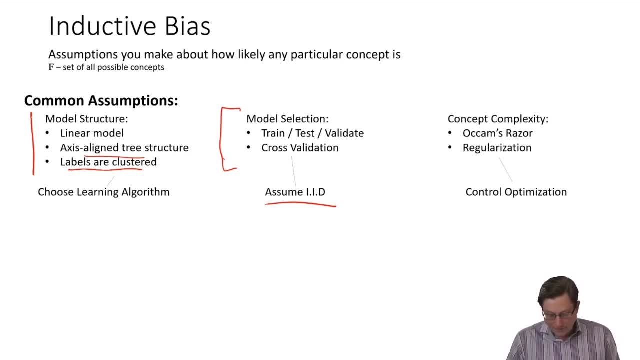 modeling process. Finally, there's this notion of the complexity of the concept. This Occam's razor is the principle that, all other things being equal, the simpler answer is much more likely to be correct than the more complicated answer. And one notion there is that you know if you have a 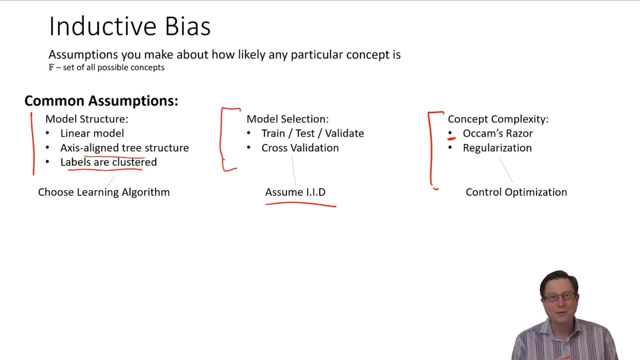 decision tree with three nodes. that is 100% right on your training data. or you have a decision tree with 100,000 nodes. that is 100% right on your training data. or you have a decision tree with 100,000 nodes. that is 100% right on your training data. you're probably going to want to take the 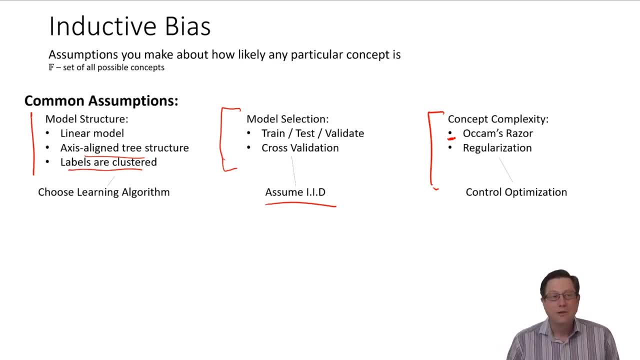 simpler one, And we'll see in a little bit how you know, overfitting is learning things that aren't really in the concept but happen to be in the data, And so using a more complicated decision tree would be more prone to overfitting. but we'll talk that through. But it is an inductive bias. 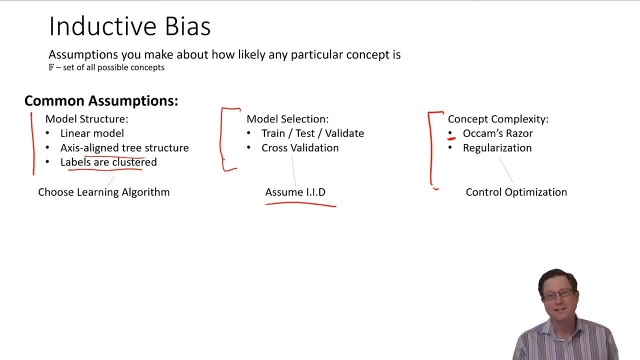 because you might know that I'm positive that there is not a simple answer to this question. So give me an answer that has at least 50,000 nodes in it, because otherwise it's just not going to be right. So regularization is a word used to talk about encoding this assumption that simpler concepts are. 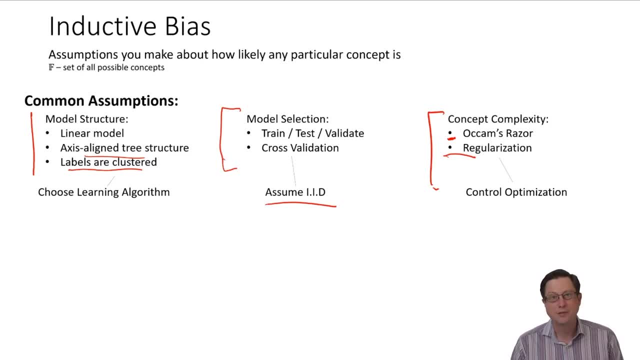 better in the modeling process, in the optimization process, so that you actually bias yourself towards simpler models and never even search for ones that are more complicated. Okay, so here is the set F, this big F, of every possible concept in the universe that could describe, that could. 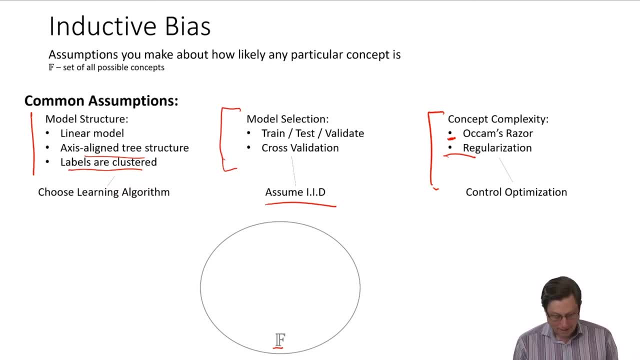 map the features of your data to possible class labels. And after you've said that you're going to set up a training process and you've gone through and written your Python code and picked the model structures, Here's the concepts that you might actually learn, And I think you know this is. 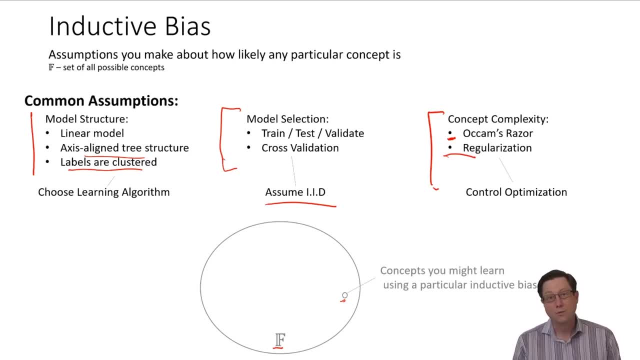 like I didn't. this is not to scale, let's put it that way- but it's quite reasonable to visualize it this way, in that your learning algorithm is only learning a tiny fraction of what's possible, but that tiny fraction would tend to be practically useful, And you know that's how you build up. 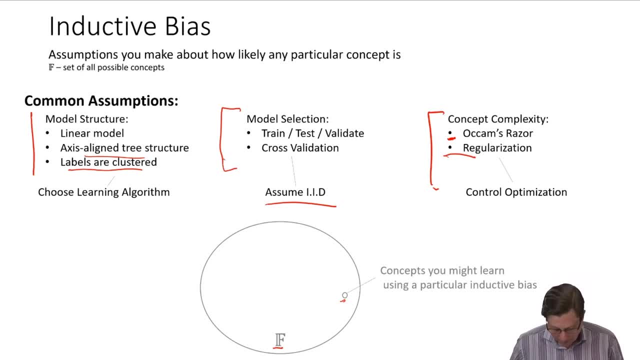 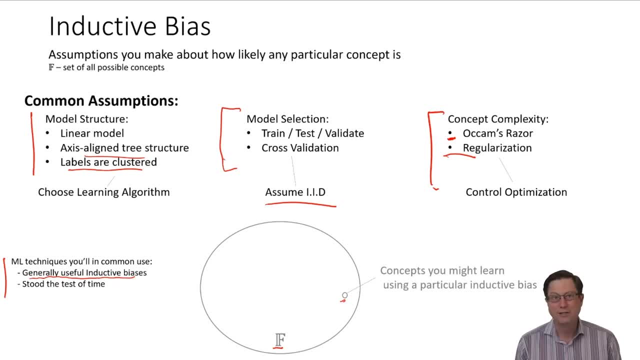 because, for whatever reason, they have generally useful inductive biases built into them. That is, they may not be the best best- best for a specific task, but they work pretty darn well across a wide range of tasks. So they are the go-to tools when you come to a new domain, And the algorithms that 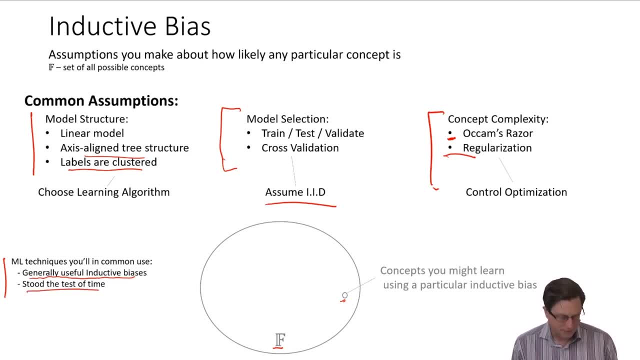 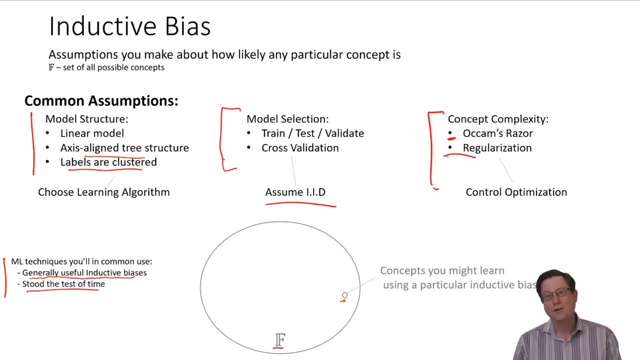 that we've explored and found the right ways to capture things that tend to happen in this universe that we happen to live in and not kind of in any other theoretical universe that might be out there. Now, one way to think about it is that stronger algorithms, more powerful algorithms, 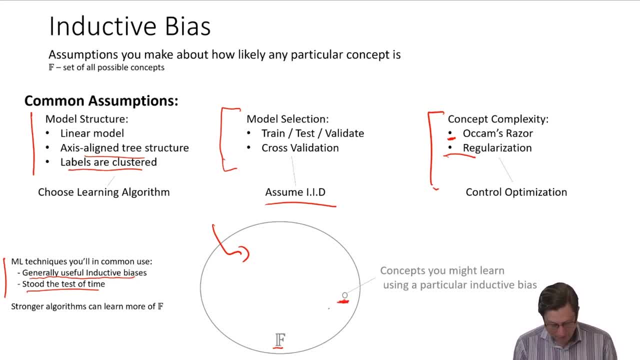 can learn more of F. So this might be the part of the concept space of all of F that you could learn with logistic regression. You might say that there's a much bigger part of the space that you could learn with a decision tree, because you can learn most of the linear concept with piecewise. 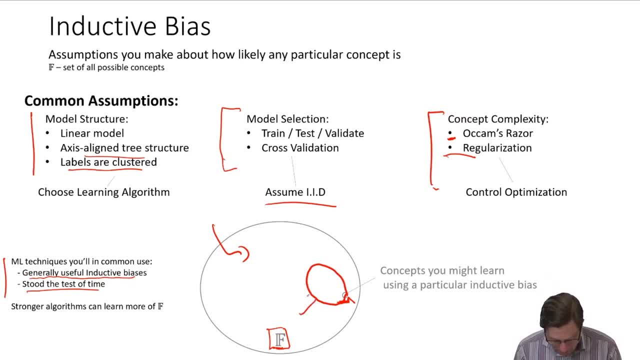 approximations of a decision tree, but not all of it. And then you can learn many, many, many things that a linear model can't represent. So it can learn more of this concept space. but that extra power comes with a cost, And the cost is that you have lost out on. 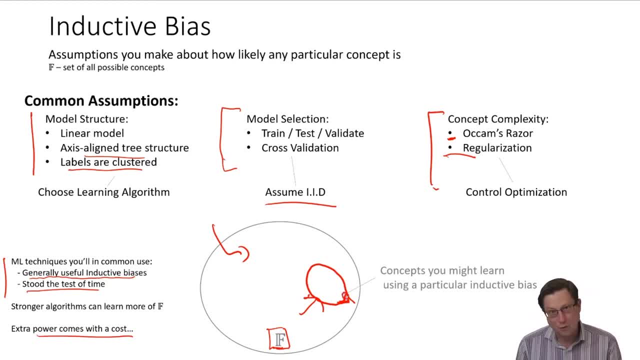 all of this, you know, focusing in on your learning process on a simple set of models. Now you have to do more to control the search process that you're doing when you look for models, so you don't get lost in this kind of like much larger possible set of concepts and learn a. 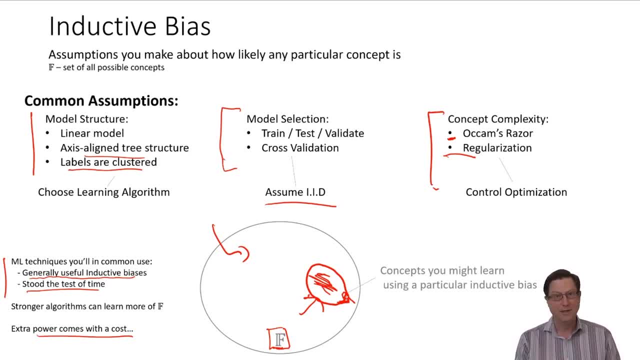 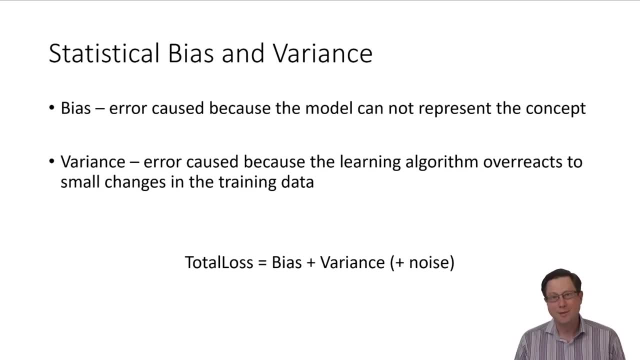 concept that is accidentally good on your training data but not good in generalization. Okay, so that is a little bit of orientation on what we're talking about and why these problems are so critical to machine learning. It's not just something that, hey, you know we're going to do. 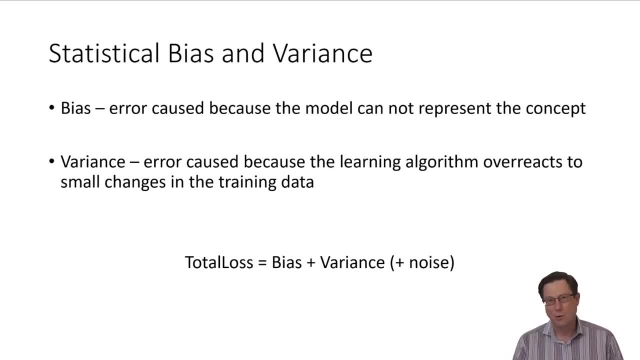 a little bit. we're going to get a little bit clever and solve this problem of inductive bias or of having a free lunch, and we're just going to find the best learning algorithm for everything. Now we're going to talk a little bit about types of errors that your modeling process can make, or 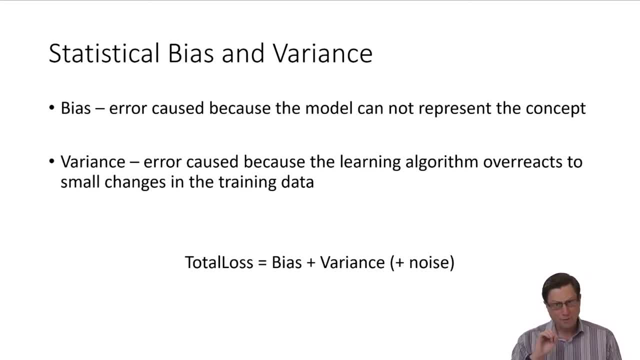 your model can make And there's. this is statistical- very common in statistics to say that there are two types of errors. There are bias errors and there are variance errors. Variance errors are caused because the model that you have cannot represent the concept at all. 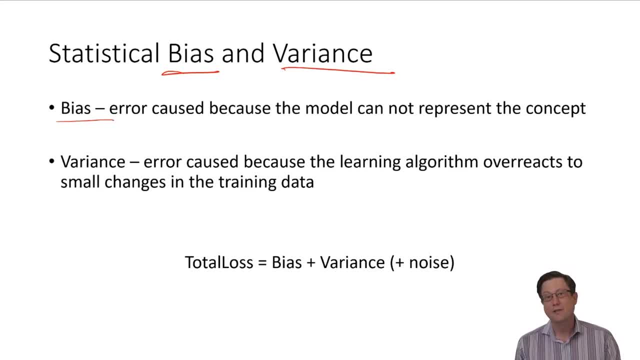 It's impossible to represent it. So every error that comes because you can't represent truth you would call a bias error. It may not be necessarily easy to measure those. There's no like pull out an error and say, well, what caused this error? But that's just conceptually. 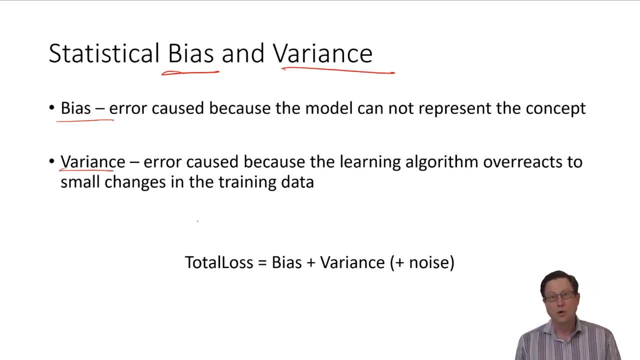 And then variance errors are errors caused because your learning algorithm overreacts to small changes in the training data. That is your learning algorithm. but also the process of hyperparameter sweeps that you've done learns a model that happens to model the training data but does not generalize well to the actual concept. 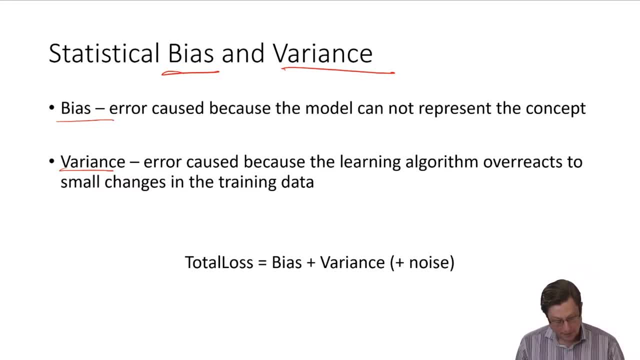 Now, a lot of what you try to do in machine learning is trade off bias first variance errors so that you make as little. you use a modeling approach that is as powerful as needed to drive down the bias errors, without being too powerful and starting to lose control of what's going on in the model, And that's what we're going to talk about today. 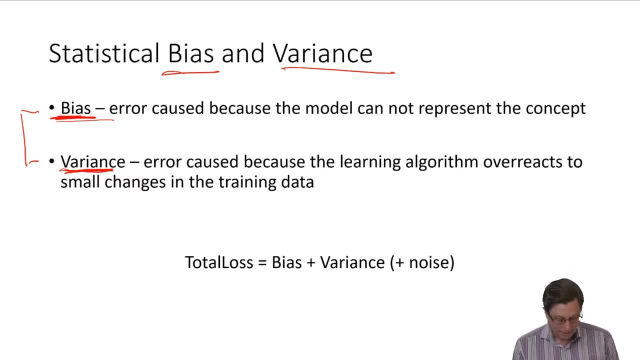 So let's talk about this some more And you can say the total loss of your learning process and remember the loss is model structure, loss search. So we're talking about that loss component, but the total loss can be said to come from the bias part of the loss plus the variance part of. 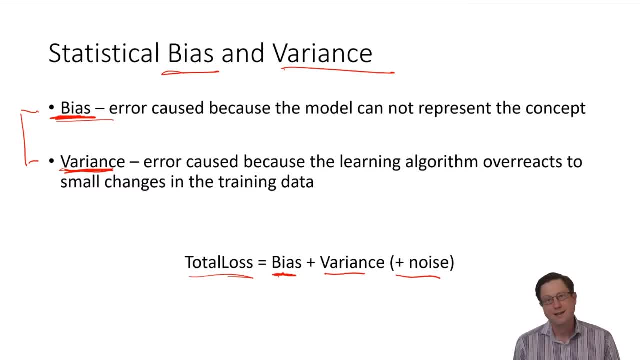 the loss plus noise, where noise is just like training. data got a little bit corrupted. Somebody labeled, hand labeled it, but they hand labeled it wrong. There was a problem in logging. I mean, there's all sorts of reasons that noise come into the process, but when you're 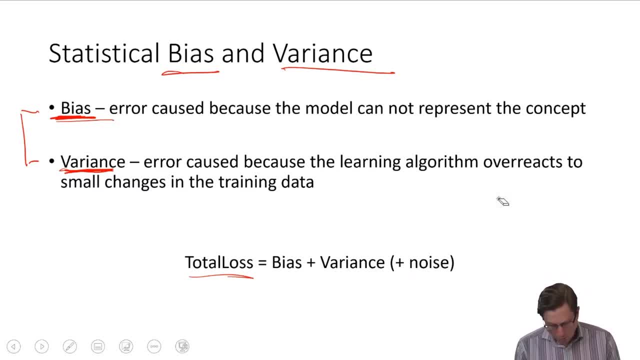 doing machine learning, you're always going to want to look at your errors and say, well, which part of this, how much of this loss that I'm observing from the current model, how many of the errors that it's making? what I say are bias, or what I say are variance, And then, by having a 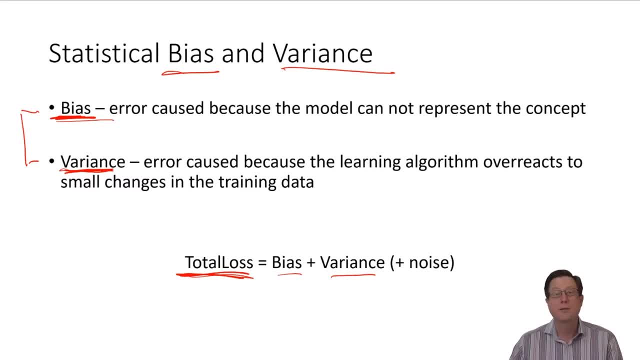 sense of that in your mind. using some of the tools we're going to talk about, to come up with some sense of that, you would know how to change your modeling process to do better. right, Like, we'll go through this a little bit more Now. let's visualize this a little bit, talk about it a 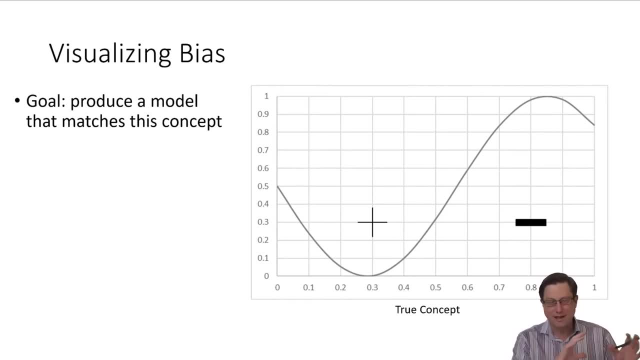 little bit more conceptually, like not with the math and the kind of like crazy concepts, but a little bit more visually, And let's visualize bias. And so if our goal is produce a model that matches this concept and the concept has X one, always label your graphs. Why didn't I label it? 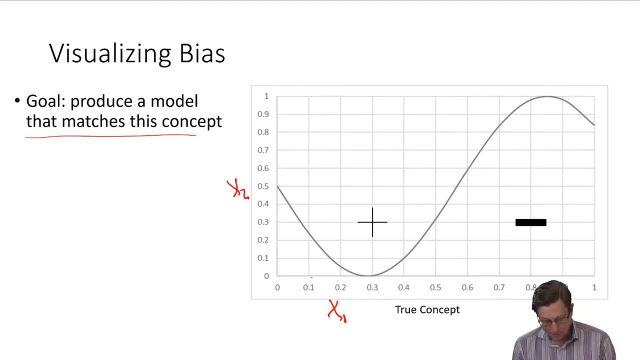 X two. I'm so sorry about that. And so you know, in this range the Y equals negative, in this range it's zero. in this range, Y equals positive. Now we're going to see where the problems can come from. So we have the training data from the concept and now we're going to do. 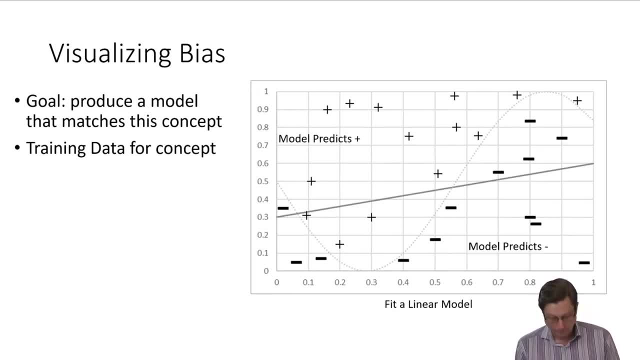 we're going to learn a linear model. There's our linear model And you can see it clearly makes mistakes. You know it's making a mistake on this. it's making mistakes there. it's making mistakes there And you could pretty much say that those mistakes that it's making are generically bias. 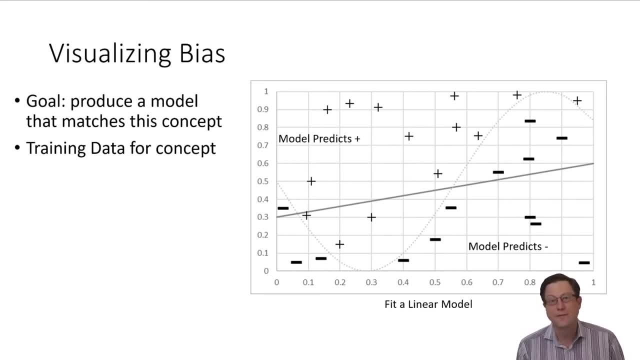 mistakes, because that's the way it's going to work. And so we're going to go ahead and we're going to call this model, you know, linear model, and it's going to represent that concept. Right there they are bias. mistakes can't represent the concept. 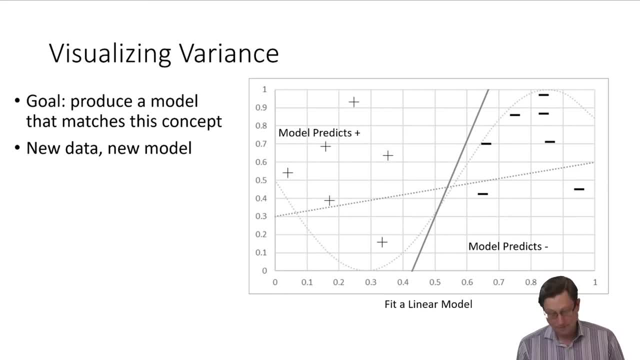 Now you could slightly tweak your training data And then you would learn a like. if this was the training data, totally different from last time, then you would learn a linear model again And you could learn a very different linear model. that linear model still doesn't correctly. 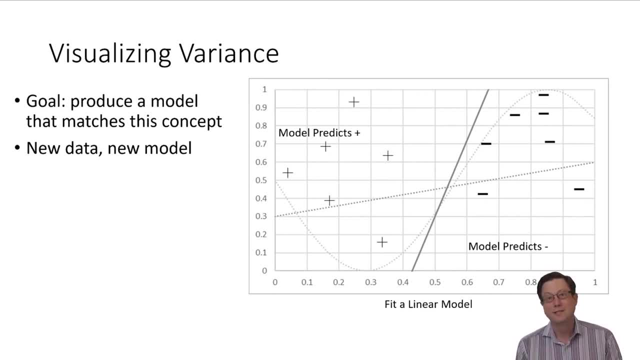 represent the problem, But it has different mistakes. In this case, the bias mistakes have moved to. you know, this region where you don't have training data, this region where you don't have training data, this region and this region, Those are mistakes. 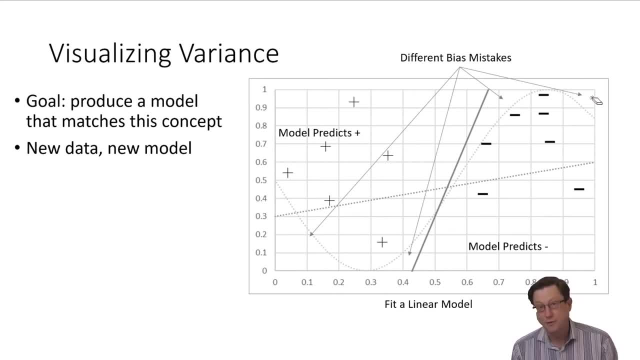 that as you try to estimate the generalization accuracy of this new linear model, you're going to find that you're making mistakes. if you have enough testing data right And they're different, you know it's different. It's going to learn the concept a different way, but it still learned it. 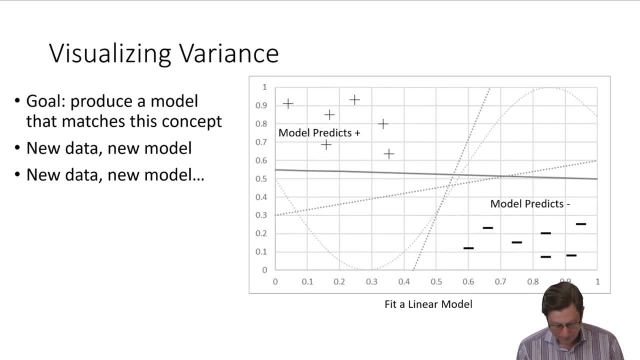 wrong And it still learned it wrong because it's not able to represent. Okay. so that was bias, where we saw that, no matter how we have the training data, a line is not going to match the concept. But variance is about the fact that every time we saw a different set, we learn the concept. a. 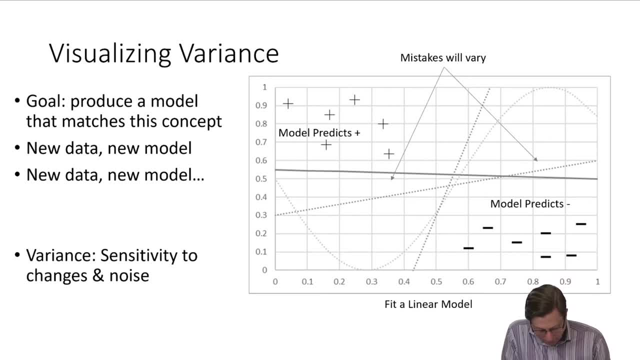 different way, And so over time you're going to learn like all sorts of different linear splits of this instance space that do the best they can on the training data that you have but don't properly capture the concept, And variance is about how sensitive. 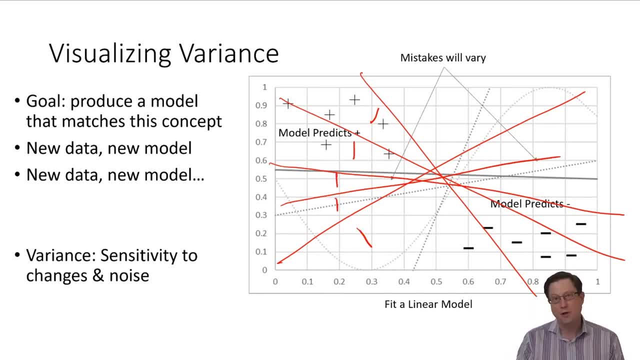 which which model it learns is to small changes in the noise. If small changes- let me just erase this stuff here for a second- So if small changes in training data means that you're learning the difference between that and that and that and that, then you would say that you have maybe. 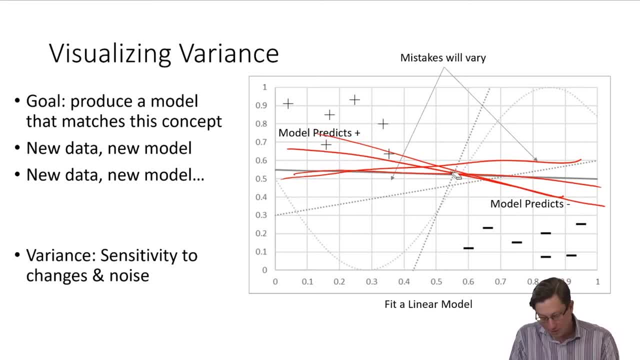 low variance errors. But if small changes in the training data can cause your model to learn the concept drastically, drastically different, then you would say that you know you're probably going to be suffering with high variance errors, And slight tweaks to the way you're using the training data could give you a very different. 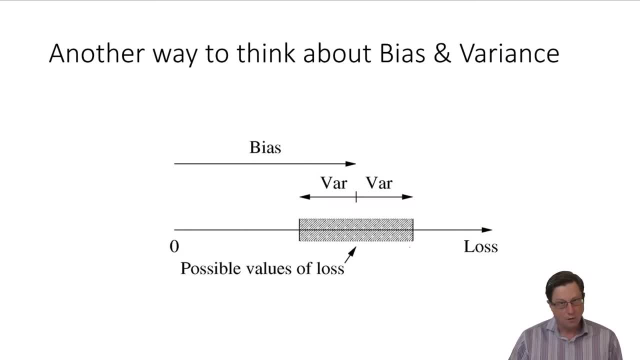 model for no particularly good reason. So there you go, a simple visualization of them. We're going to go through a few more visualizations, But I want to take a quick aside and say that here's- here's the loss from zero when you're completely perfect at the training data. 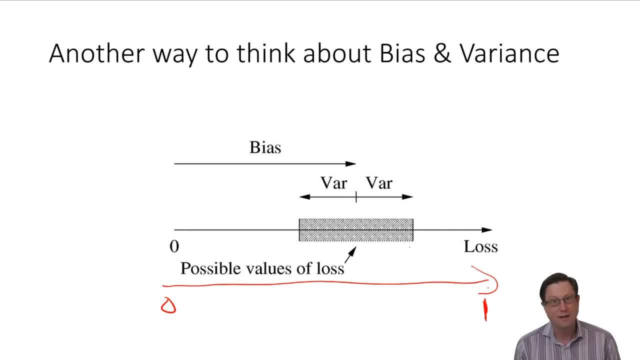 generalization data to you know the highest possible loss that you could have. And one way to think about your loss is that the bias is just loss that's built in because you've built a model that can't represent the concept. So your loss might go from zero up to, let's say, 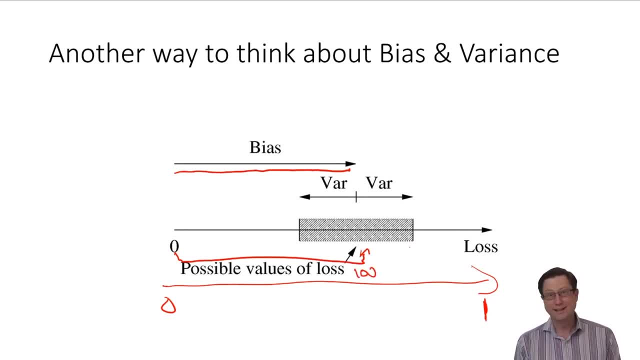 100. And you're really never going to get less loss than 100, no matter how many times, no matter how much data, no matter whatever. you don't have the right features, you don't have the right model, you have a bias for that concept. The variance errors are going to be like: 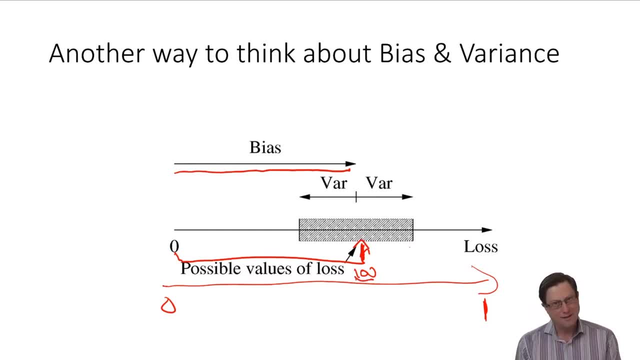 as you're trying to figure out, is my bias loss 60 or 80 or 90 or 42 or 76 or whatever it is? and you're changing small things. you're doing cross validation and and learning the model on different subsets of. 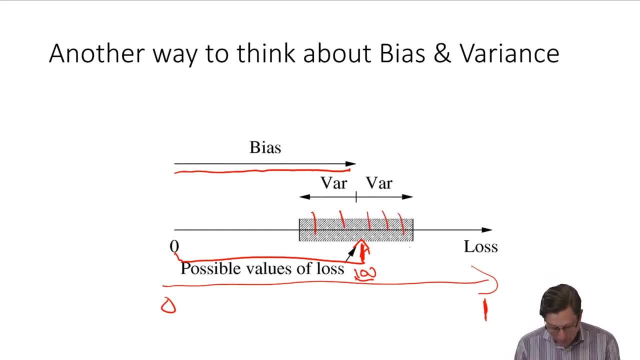 the training data. you're going to see your loss measurements bouncing around within some region that is plus or minus the loss that's caused by your bias, where you know. sometimes you'll happen to look a little bit better on the training data, sometimes you're going to look worse. but 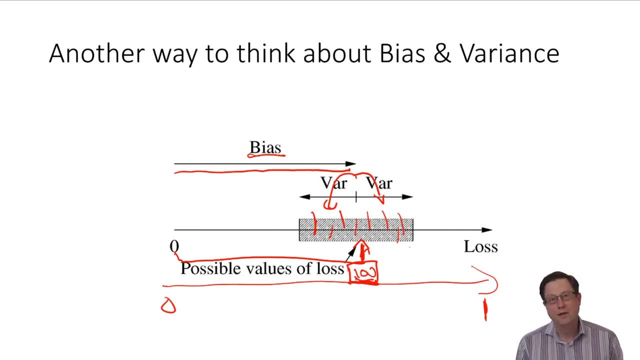 no matter what the case is, the loss can be thought of as broken down into these two components, And this is one of the reasons that, as you're doing a bunch of training runs, as you're sweeping parameters, you can look at the outputs that you're getting and you could see: hey, do those outputs seem to? 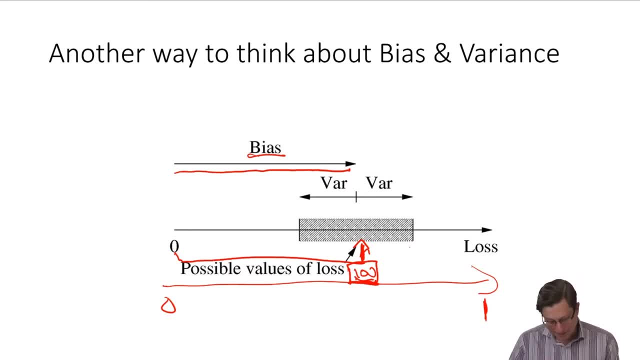 be pretty smooth When I, when I'm tweaking a parameter, is it a very small change in loss? Or, as I like, move from fold to fold of the cross validation? is the loss really jumping all over the place? And this is the first step towards getting intuition of looking at all those stats. 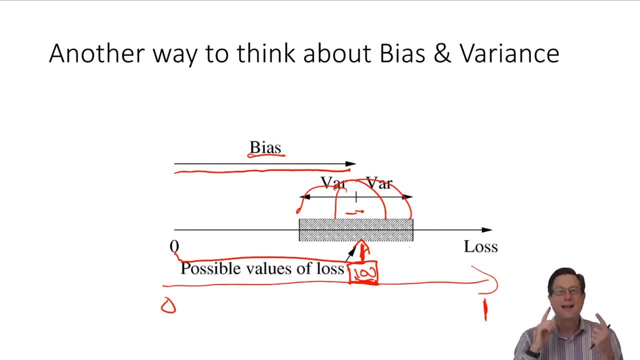 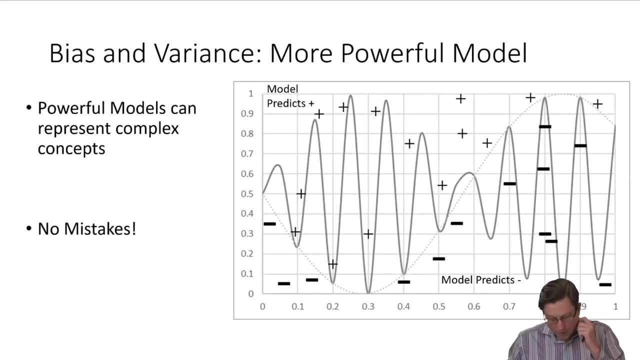 that come out of the training run, and then looking at the loss that's caused by the loss. So here's another example to say: well, of course you know we're trying to learn a sine wave here. Linear model's not going to learn it, of course, but there's plenty of other models that you could. 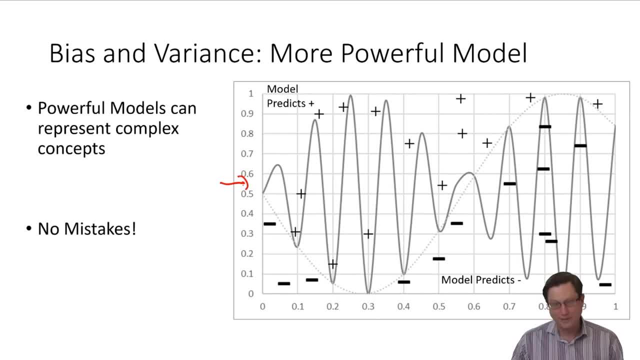 use, And here I've tried modeling it with a high order polynomial right. I don't know So, but the you could see that the true concept up here is plus the true concept on this side of the sine wave is negative. I'll draw the sine wave again so it's a little easier. 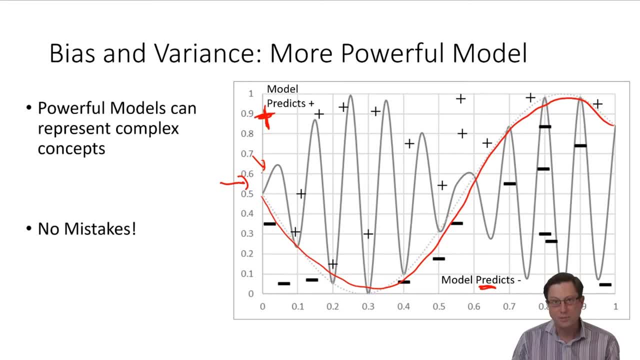 to see. And then you learn this high order polynomial on your training data and it wiggles all over the darn place. It's learned the concept kind of like incorrectly, like super incorrectly, because it thinks that this part of the instance space is minus and this part of the instance 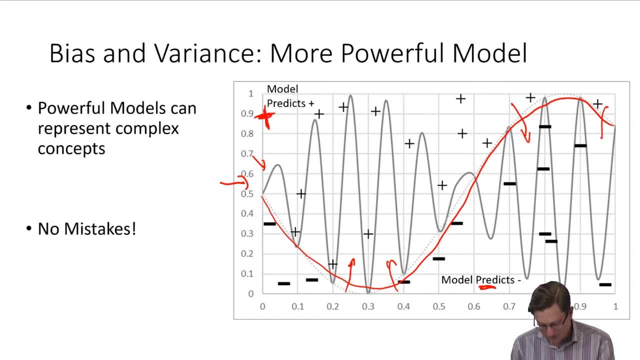 space is minus and this part of the instance space is plus and this part of the instance space is plus. With a high enough order polynomial it fits all the training data. You can fit any actual training data with something like this, but it fits it in a way. 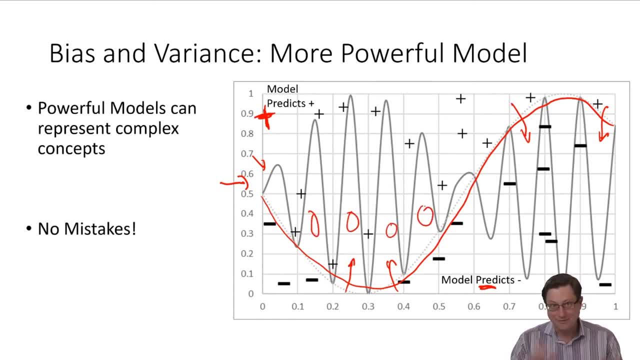 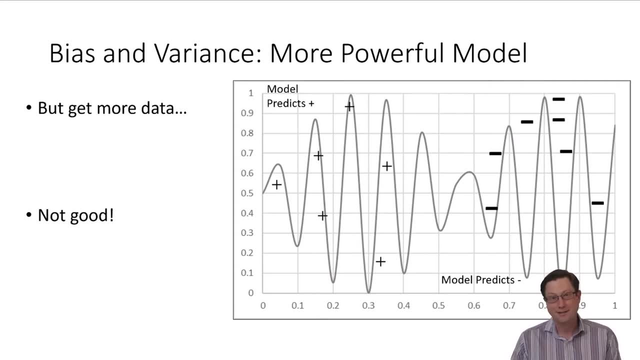 that makes tons of mistakes just because of you know, it's just oversensitive to what's going on. So now, if you get a different training set, slightly different training set, you just you go to your validation data and you could see that this one I'm pretty sure I mapped it out. 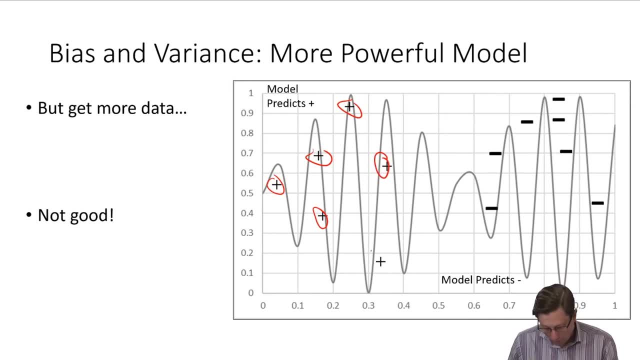 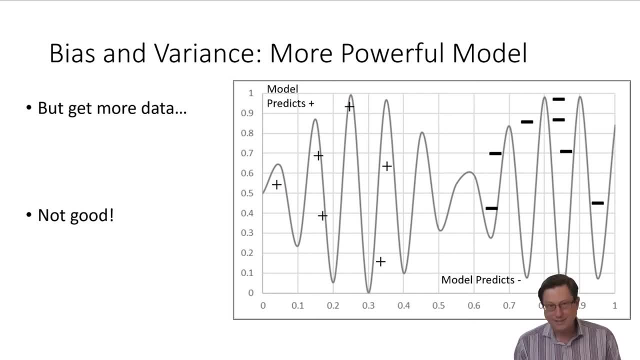 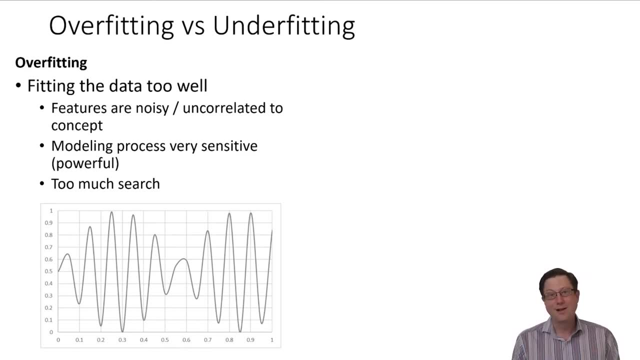 you will. I don't think I ever have, But that's not good. So for a little bit of a summary, when you're doing machine learning you're going to have this constant balance between bias errors and variance errors. Bias errors come when you underfit the concept, that is. 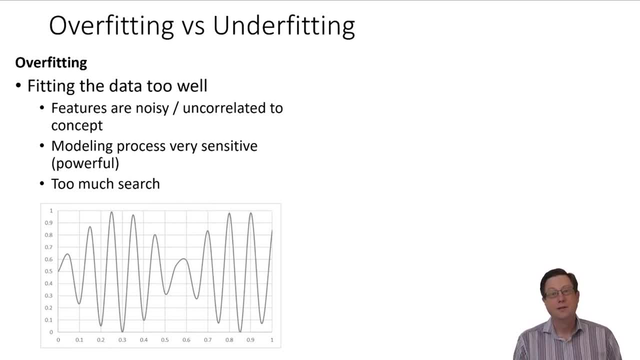 when your model is not powerful enough, And variance errors come when you overfit the model or when you're too responsive to small changes in what's going on. All right, so to say it again: right, like overfitting happens when you fit the training data too well, when your model is so powerful that it can find a 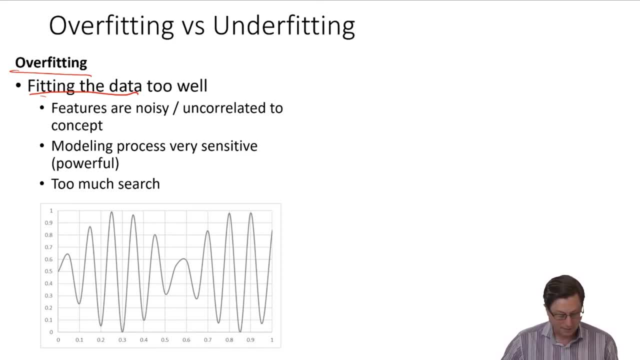 way to fit that training data, even if that has nothing to do with the underlying concept. And overfitting can occur when your features are noisy. For example, there's a feature that's completely random, It has nothing to do with your true concept, but there's just. it's a number. 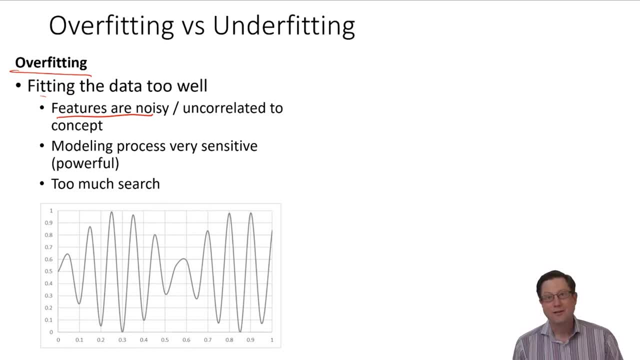 And eventually, if you know there's enough, if the randomness in that feature is proportional to the number of training datas, you might have the case where your model learns: hey, I'm going to only look at that feature, that's random And I'm going to you know if it has random value 1,. 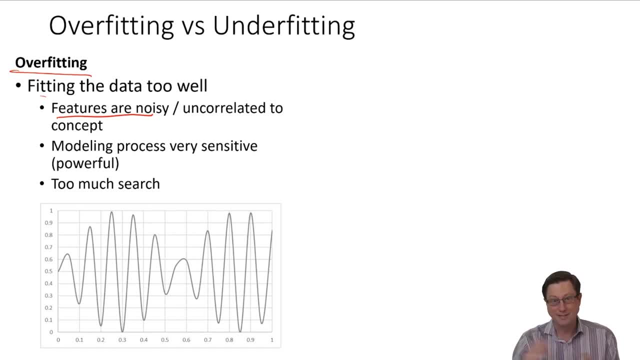 I'm going to predict 1.. If it has random value 47,, I'm going to predict 0,, because that's what's in your training data. So then you're overfitting to that feature, which has nothing to do with the. 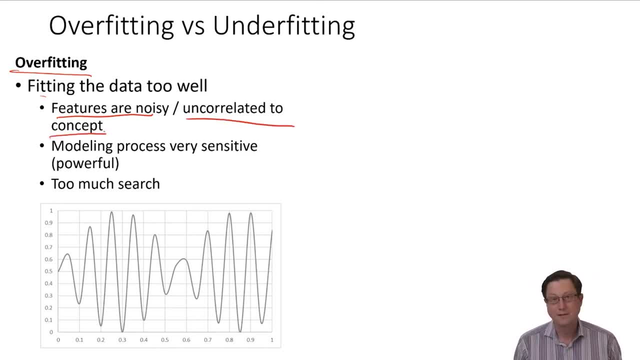 concept Completely uncorrelated to the concept that you're trying to learn. So that's one way that overfitting commonly happens And it really requires also that your modeling process is powerful, And powerful here could be. so you could think of it as a proxy for the number of 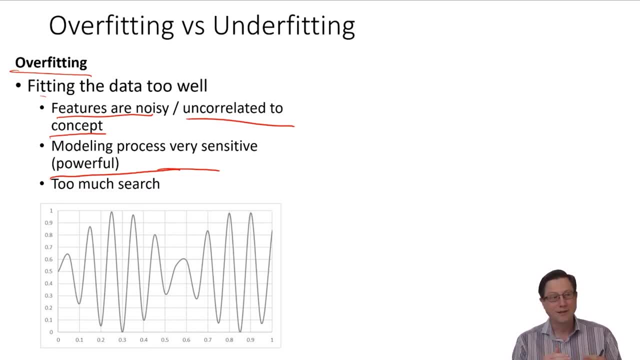 parameters that your model has or can your model's like? can your model's number of parameters grow unbounded, as it's processing training data, as in decision trees or, you know, with neural networks? you might try to learn a neural network that has a billion parameters And you're 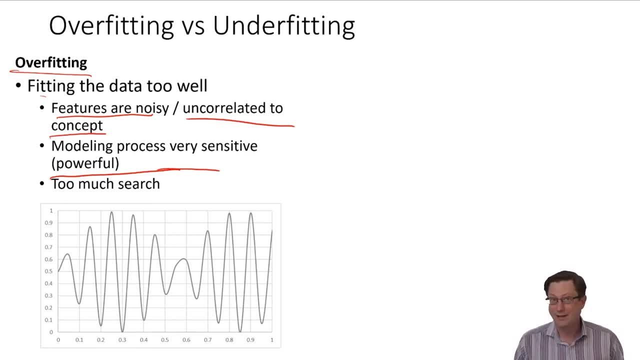 going to have a lot of parameters in it, And that's a lot of parameters. That's a great amount of power. It can create very complicated models, But it's also highly prone to overfit, So you're going to have to do a lot of work to avoid overfitting when trying to learn that many 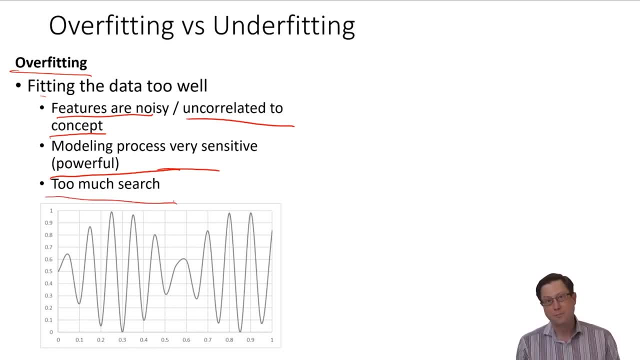 parameters. And another way to think about the power and the parameters is the hyperparameters that you use. that can control how much search you allow the modeling process to do. If you tend to cut off search early, then you have reduced the ability, you've reduced the opportunity. 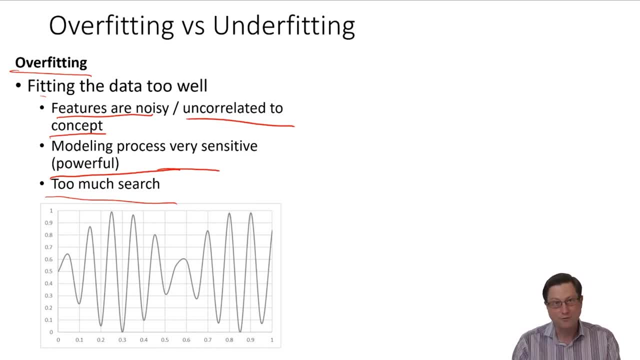 for your model to overfit because you haven't allowed it to go too far, Whereas if you allow the model to just search and search and search, eventually you are going to possibly start overfitting. if your model is powerful enough to overfit the data Now, underfitting means that you 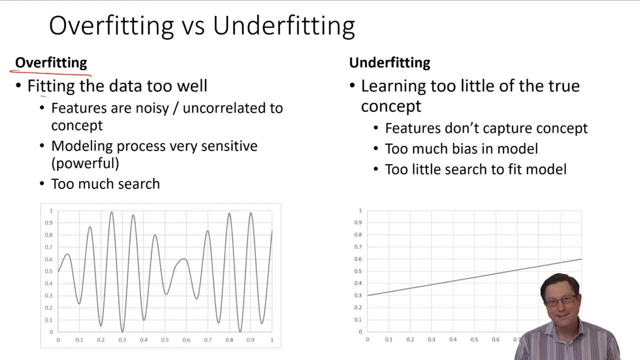 have failed to learn the true concept And you could say that these are bias errors. They're biased either in the model structure, where you're trying to learn a linear model for a complicated thing, Or they could be bias errors, either in the model structure, where you're trying to learn a linear model for a complicated thing, Or they could be. 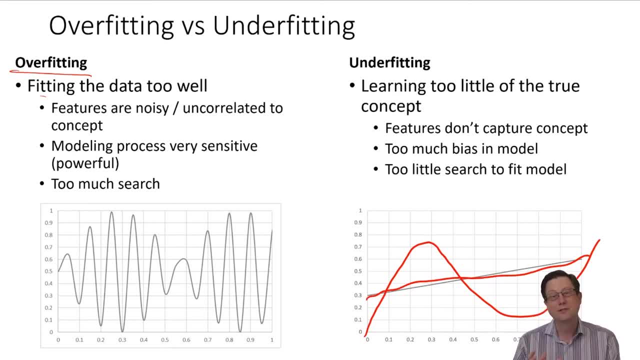 in your modeling process where you didn't allow enough search or enough time or enough training data for your model to go ahead and figure out what you're trying to learn. so there's, you know, bias in the model structure itself, bias in your modeling process and when you have high bias. 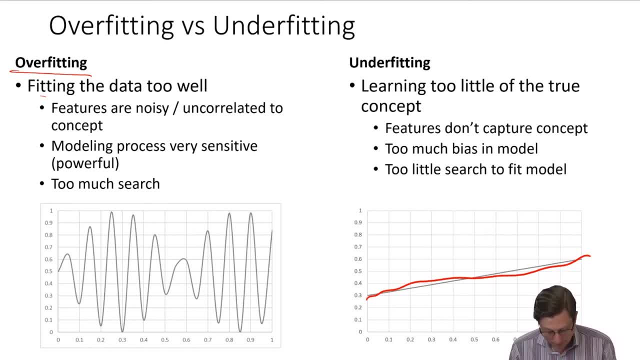 errors. it's said that you've underfit the concept. now let me just read through these. you've learned too little of the true concept, and this could happen when the features don't capture what you're trying to learn at all, which means if you've done feature engineering and you've 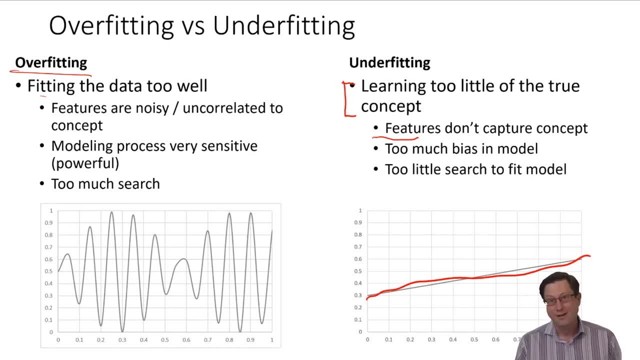 created a whole bunch of features that have nothing to do with the concept you're trying to learn. you're not going to learn the concept right, even no matter what right that's a. you've sort of thrown it out because of your choices with feature engineering. you said i'm only using two features. 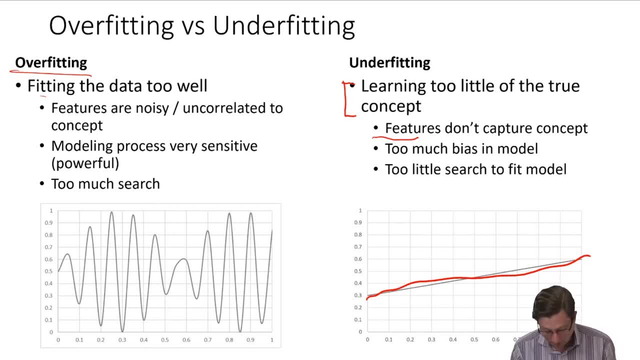 well, you might have a hard time learning like something that's interesting or complicated. another is that the model type you've picked has too much bias with respect to the true concept, as in the case with this linear model here. when you're trying to learn, you know la-di-da. 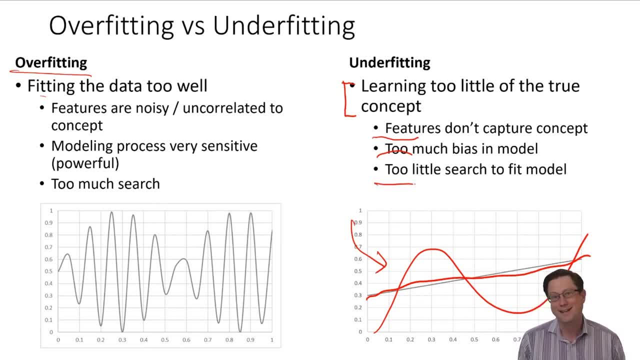 and then you know you could have a modeling process that does not allow you to get where you need to get. so even if you are learning a high order polynomial with enough constraints that could actually learn that, but you've only allowed it like 10 iterations of gradient descent, something along those lines. you may not, you may, you know you may end up. 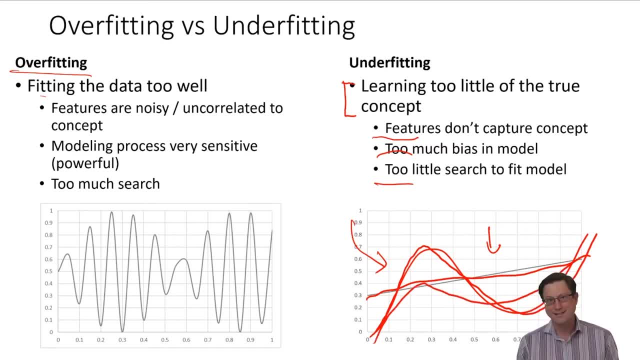 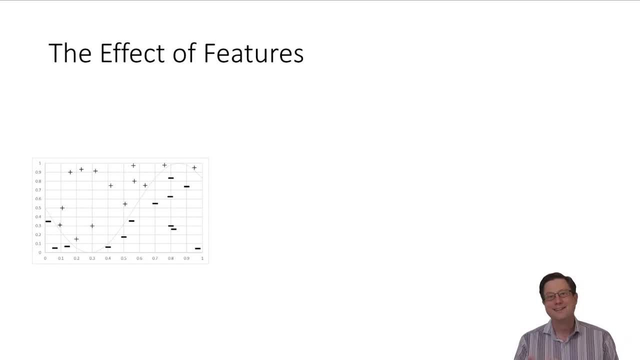 learning something like that and 10 iterations of gradient descent is not enough to ever get you to where you need to be, and because of that, your modeling process is leading to underfitting. all right, so you know, on that last slide, i said many, many words, i had lists, lots of stuff, blah blah. 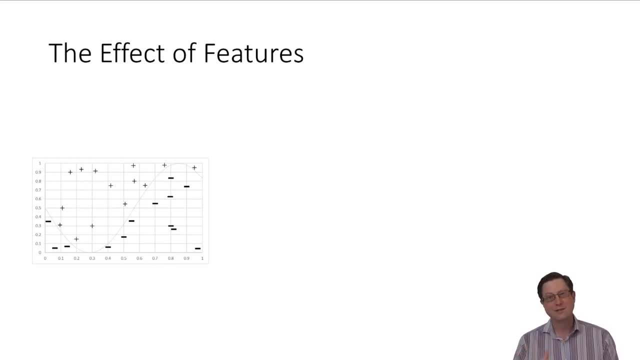 and i'm going to go through one of those sub bullets in a little bit more detail just to give you more time with this concept, to give your brain some time to stew in it and and start to make these connections now. first of all, this is the example we've been showing and remember: label your axes. 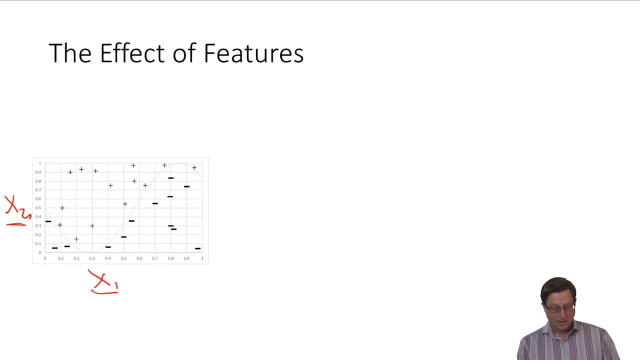 label your axes. but this is what we're doing, and so what these features do is they expose parts of the concept to your learner. now imagine you did this differently, where you didn't have x2, all right, so you've thrown away x2, you projected everything down on this axis, and what's going to happen? well, it's going to be. 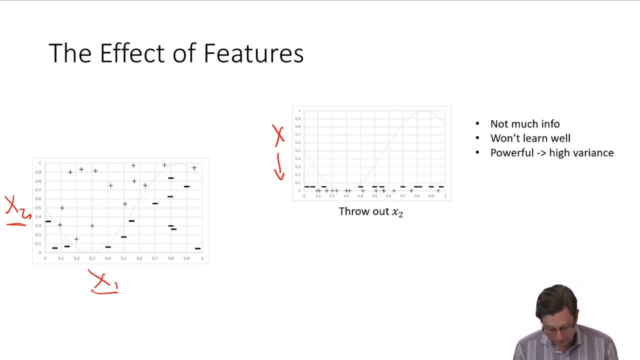 harder to learn, right, you're going to have a hard time learning this concept, for the data you could see, you know this. this sign is near there. so in this range, almost everything is going to be plus, and in this range here, almost everything is going to be minus. but in this range, here it's going to. 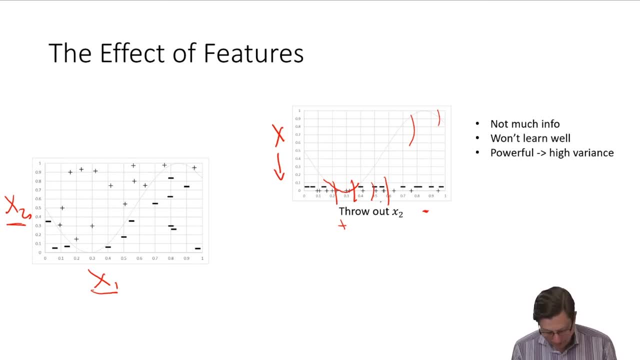 just be 50- 50.. so you pick a sample with an x1 value in that range and you might as well flip a coin to get the label, and so what that means is that you're not going to learn it very well because it's you know, the concept isn't exposed, but if you do have a powerful model that is able, 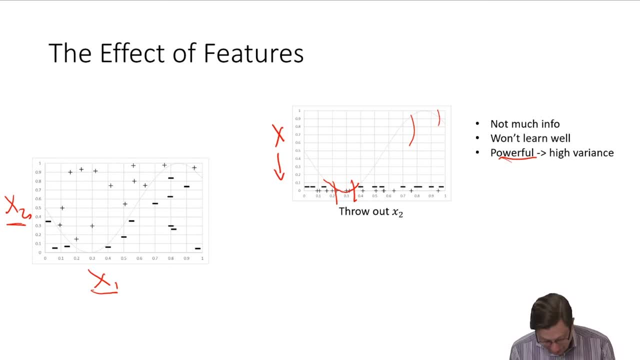 to learn these variations, like in this range. it's going to heavily overfit the training data because the label is really sort of uncorrelated at that point. it's like a coin flip away. um, so you're gonna, you know, you're gonna- learn a whole bunch of like, splits, like that, if you're learning a decision tree, something along those lines. 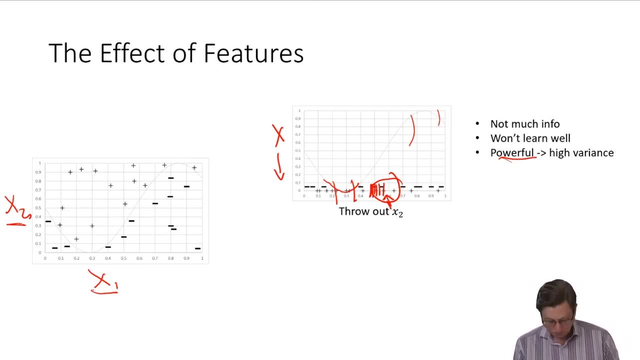 it's just because the concept isn't there for you to get at um. on the other hand, if you're really good at feature engineering and you're like, hey, x1 and x2, those are all nice, but they're not what. they don't have anything to do with the concept. but 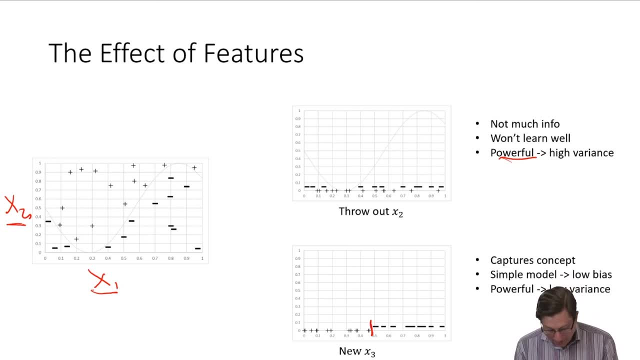 you actually know what's going on and you add a new x3 that projects the whole thing onto another dimension where there's a very simple answer. x3 contains the answer. great work, you've done beautiful feature engineering and so this captures the concept and a simple model can learn a very low bias representation of the data just by only considering x3. 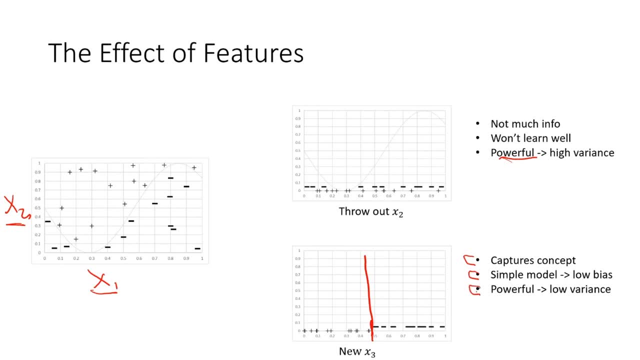 um, and a powerful model will have low variance because there's nothing for it to overfit. you know, everything over here is looking good. everything's over here is looking good, um, so you can be in great shape, and this is just to say that good feature engineering can get you. 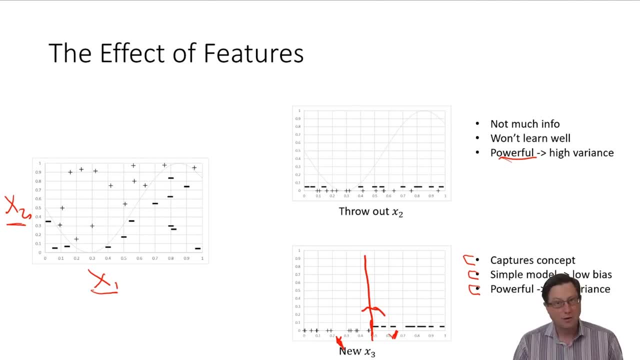 a long way and that modeling power, modeling process, etc. etc. all the downstream stuff i mean. they're. they're all good, So I think that's all related. doing poor at any spot along the line will lead you to have errors that you will see as bias errors or see as variance errors and need to correct and you'll need to like, say well, 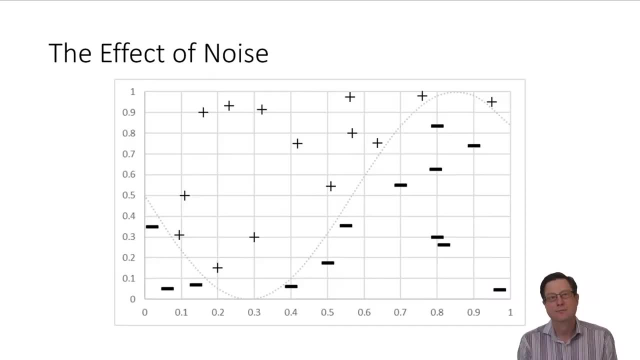 where is this error coming from? it could come from many, many places, all right, and i'm going to do one more example. so that last one was the effects of poor feature engineering and outrageously good feature engineering. now. the effects of noise, um, you know, like we said before, we could learn a. 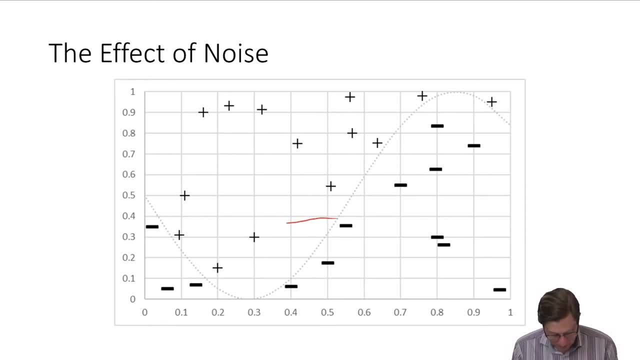 decision tree for this that approximates. you know, do a split there, then we do another split there, then we do another split there, and so you know it's saying: well, that's minus and that's positive, and then we maybe we need some more splits or whatever. but okay, fine. 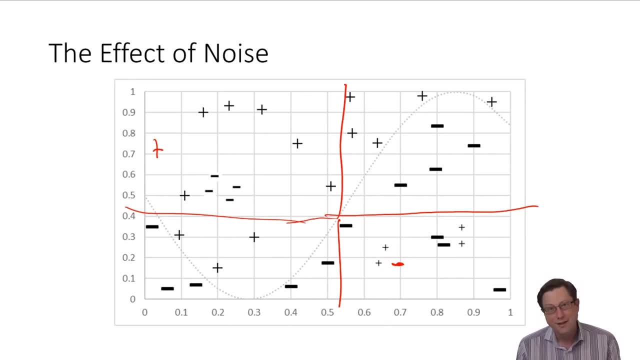 so we have a decision tree. it's sort of learn the concept. but what if some samples have noisy labels? now a decision tree can learn those noisy labels. it can say, well, oh, let's cut this region off and let's, you know, do another set of splits there. you know, i guess they'd look something more like this. 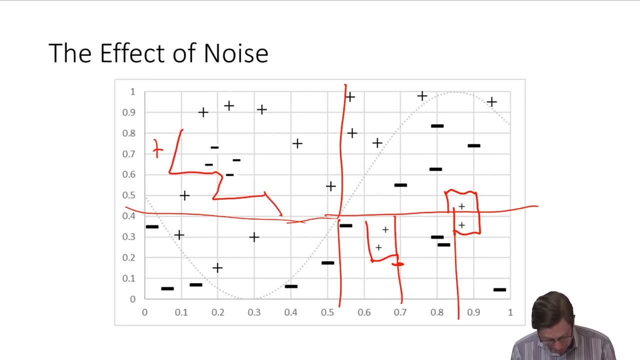 but you'd split those regions off and then it would learn like a whole bunch of splits to carve this region off and it would say: you know, everything in here is minus, everything in here is plus, everything in here is plus. and where does this noise come from? who knows it could be. you know your users got. 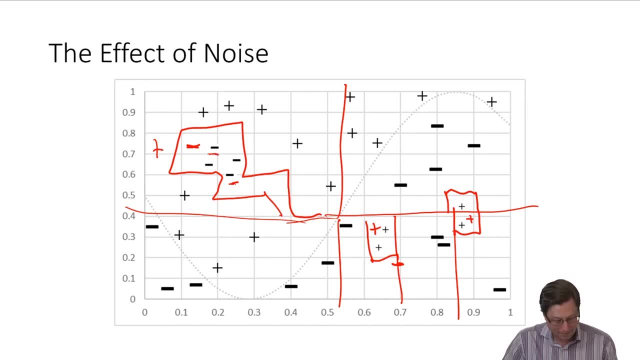 confused when they were giving you a label. or could be you paid somebody to hand label this stuff and they got bored. maybe they fell asleep on the keyboard. a little noise like this can lead a too powerful modeling process to really pick up on some gibberish and come up with 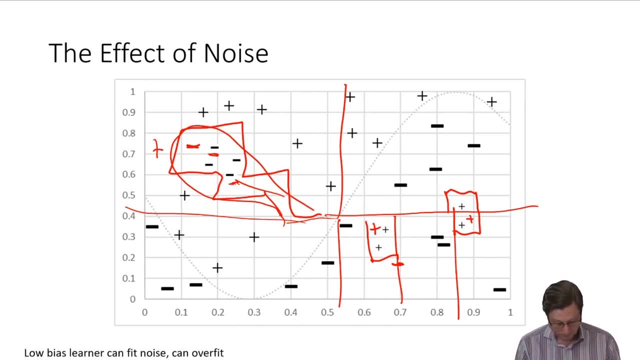 something that has nothing to do with nothing, just because there's a little bit of noise. now you could just to belabor this point. a model that is not super powerful, like a linear model, really can't address this noise. it has no way to chase that noise. it like having these samples. it. 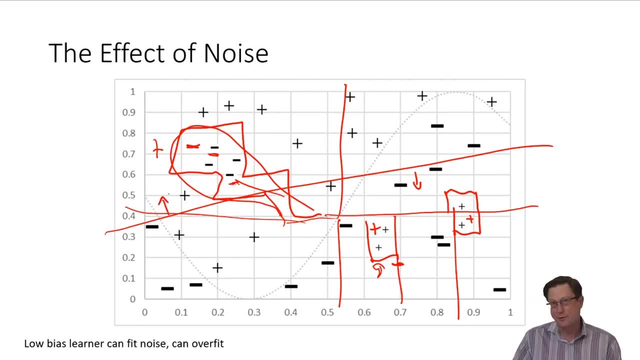 might shift the plane, that it learns a little bit in that direction to, you know, to minimize loss a little bit differently. but it is not going to have the same level of overfitting problem as a more powerful model that generally you would say: well, it has a lower bias, that's. 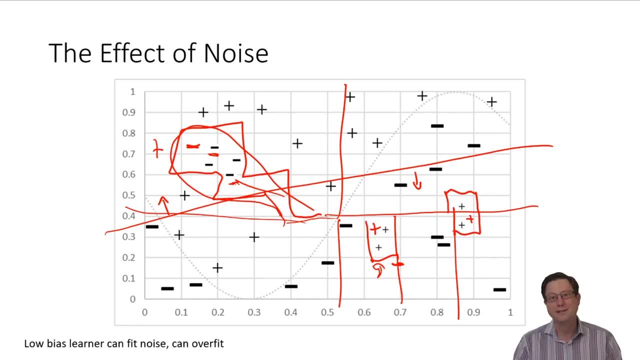 better. but no, it can chase this noise, it can chase this problem and it can get itself into trouble. so just you know multiple examples of how this bias variance thing is going to be a trade-off: overfitting and underfitting. are you know they're gonna both happen. um, and some sense of what leads. 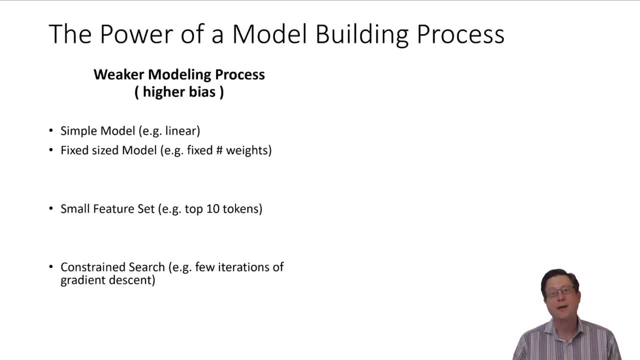 to them. okay, so what do you have to do? you have to think about your modeling process and how it's going to interact with bias or variance errors, and if you need to get rid of variance errors, you can trade off and increase your bias errors to get rid of some variance errors, and one way to do that. 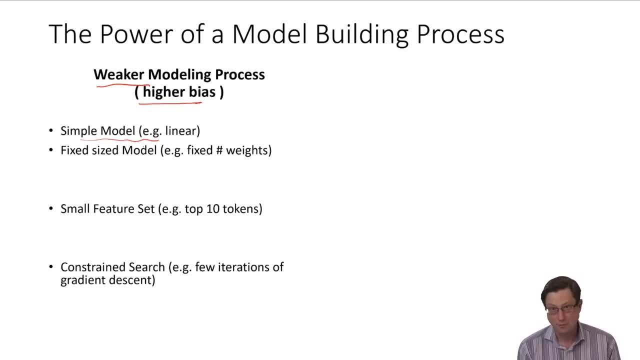 is to move to a simpler model, for example, logistic regression versus decision trees. another is you could have a fixed size model, that is, you could change the parameters that control your decision tree learning process so that you just can't learn a bigger model. another is that you could 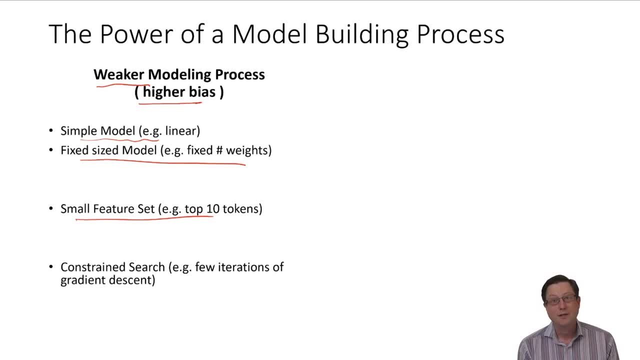 do more feature selection, throw away features, spend more time maybe in the wrapper method to find ones that really suck all the information out of the feature set that you have. and then also fixed size search, and it's a little bit of a duel with the fixed size model. 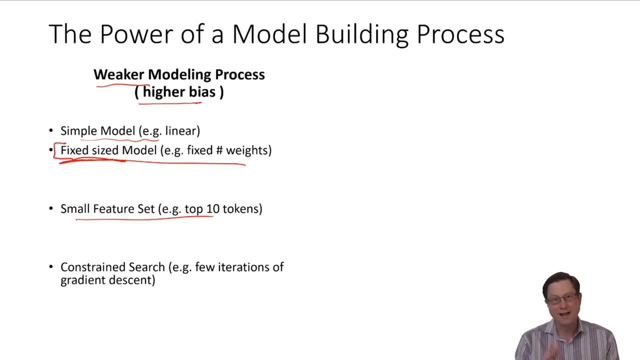 because sometimes the model and the search go hand in hand. but even when you're doing gradient descent or something along those lines, you can do fewer iterations of gradient descent or put other controls on the gradient descent that keeps it from going as far as fast, so that you are less likely to overfit or highly fit the training data that you happen to have. 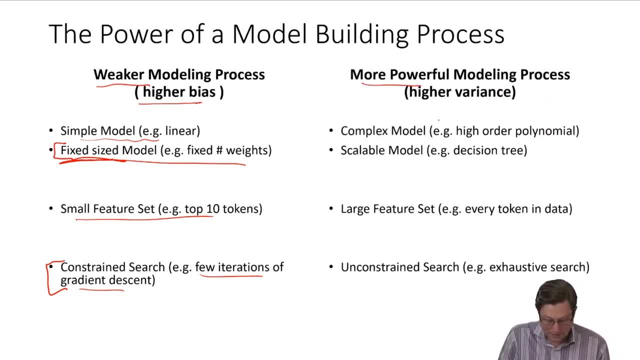 now, a more powerful modeling process is what you'd want to use if you're willing to take more variance errors in exchange for having fewer bias errors, and so if you think you're in the place where you know your, your bias is killing you. you could use a more complex model in our previous. 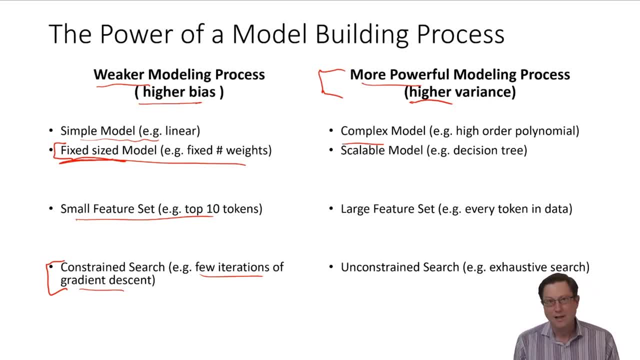 example, it was, like you know, higher and higher order polynomials, but this could be like decision trees or boosted trees or neural networks or neural networks with more neural network structure or even adding more features- really throw the kitchen sink in terms of features at the problem. even a linear model can be quite powerful, as 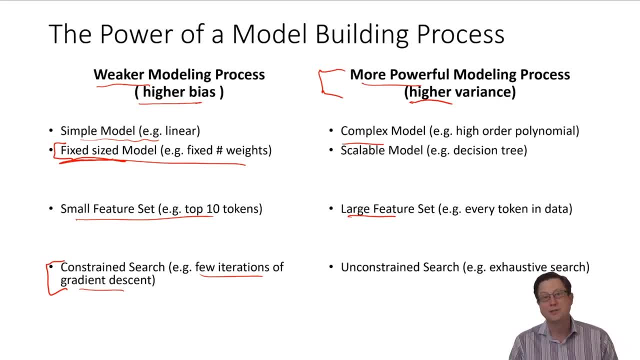 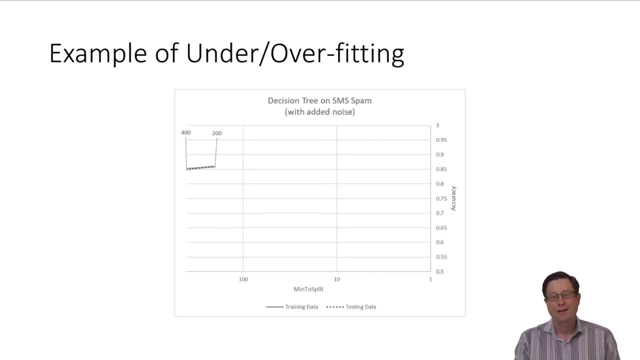 until you really do fit that training data as well as you can. okay, now here i'm going to show you the types of things that you're going to see, the types of data you're going to see coming out of your modeling process that you can use to make better decisions about which hyper parameters 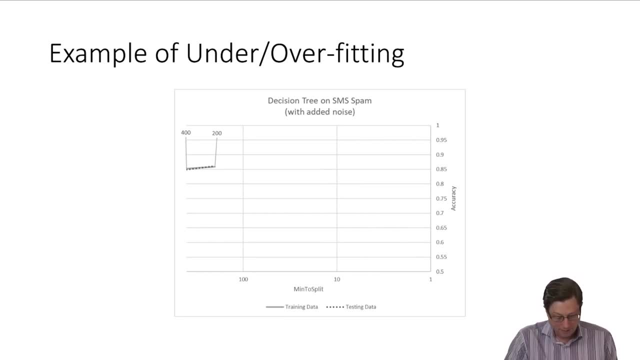 to explore and where you are in this bias variance trade-off. now let me explain this graph for a second um. on this axis, you have the accuracy of the training data and the testing data, or maybe we should say validation. you know whatever, whatever set you happen to be using and 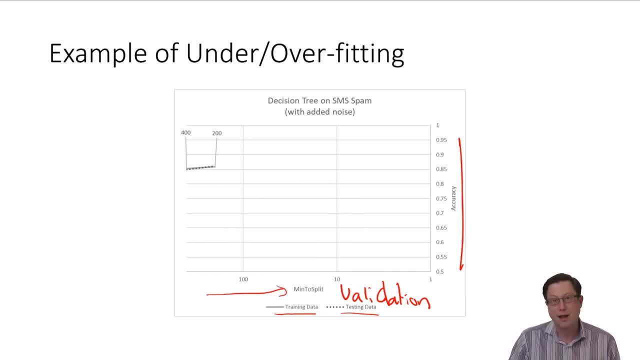 this axis. we're talking about the min to split parameter, and that means, in order to add more structure to your decision tree, you need at least 100 samples to to split, or 10 samples or one sample. these two points here are for 400, values of 400 and 200 to the min to split parameter. okay, so, 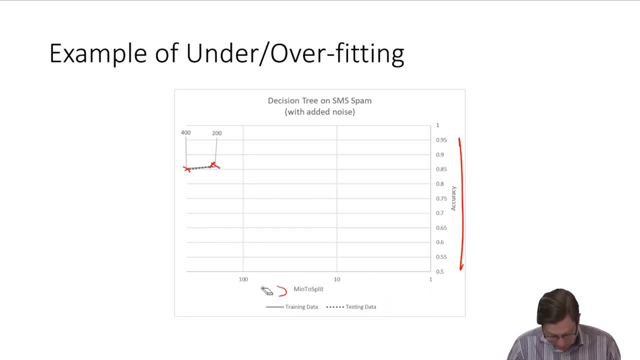 that's just to orient you on this chart, and so what you can see is that when you're using min to split the range of, you know, 200 to 400 or something along those lines, the accuracy on the training data and the testing or validation data is very, very similar, and that means the amount of concept. 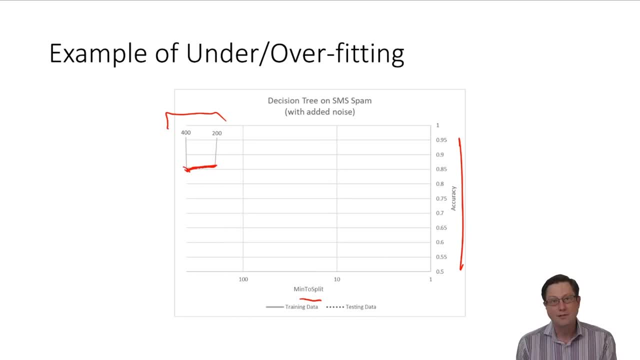 you're able to learn on the training data is translating very well to your estimate of your accuracy on your testing data and and that's in some sense it's a good sign. but you could see that going also from 400 to 200. it seems that things are better now. i haven't drawn error bars. 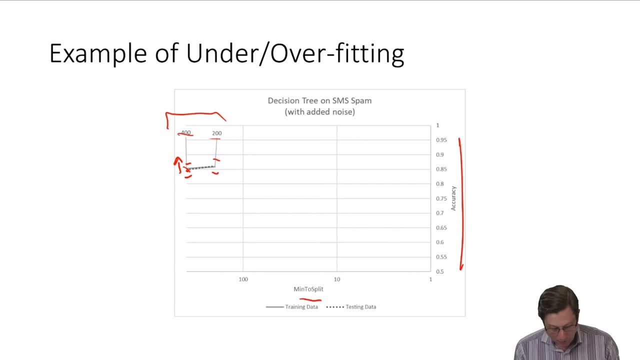 you could draw error bars and maybe you'd say, well, it's just noise. but a lot of times when you're doing a parameter sweep, the noise on a particular point is interesting, but also the trend is very interesting. so even if you see something like this, where these guys look to be within the noise of 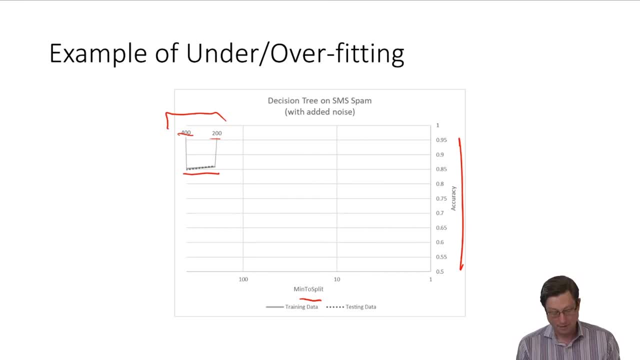 each other go ahead and measure another parameter, another value of this hyper parameter. so let's try something a little bit further now. i've tried two more, we've tried 100 and we've tried 50. now you have a couple interesting things now when you look at this chart. first of all, the training accuracy. 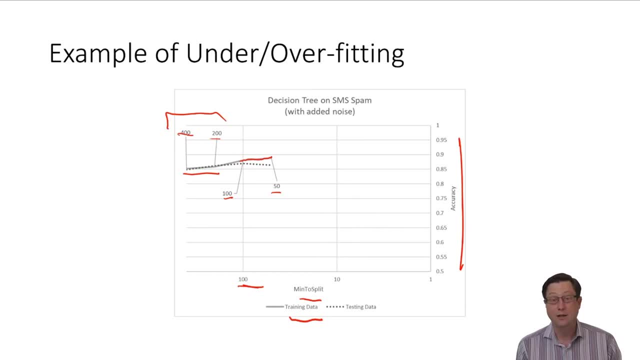 has continued to go up and if you're looking at the training data alone, you might be saying, wow, this is heading in the right direction. you may have started to, like you know, if you have some error bars there, this value might be high enough so that these, these um confidence intervals, no. 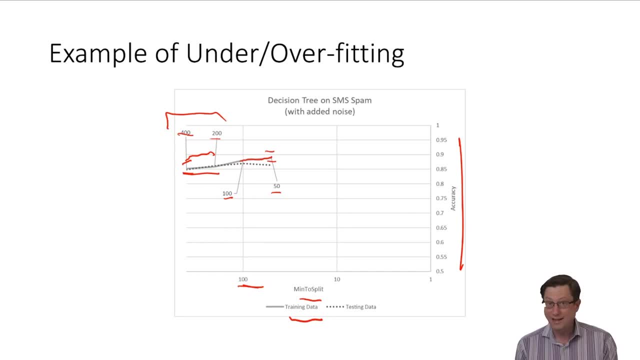 longer overlap and you might say that, hey, with 95 confidence on the training data, using 400 as my mint split is significantly worse than using 50 as my mint split. that's perfectly great. but look at the test, the testing data. now they're starting to be a problem because 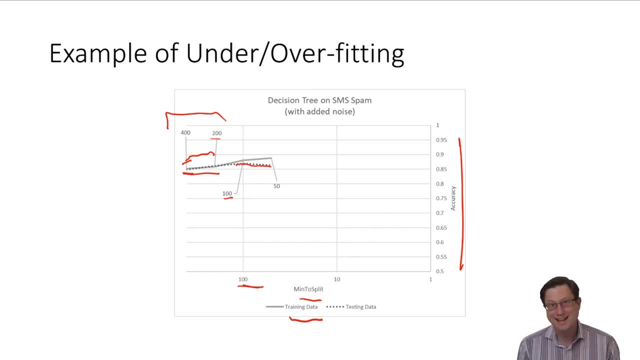 the accuracy, the generalization accuracy on your testing data is no longer going up at the same pace with the accuracy on the training data, and so now you've got to say something might be going on here. things are small. this difference is small, so if you're doing error, bounds on everything you might. 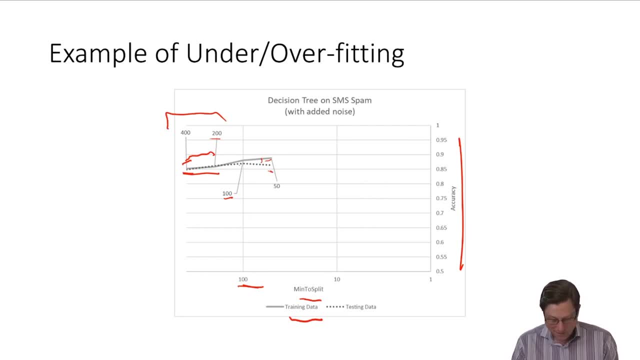 say like i don't know, yeah, i mean it's, it's not super unlikely to have a reading that that. that's that different between the training data and the testing data. that might just be noise, okay, whatever, we'll use the error bounds and we'll ship okay. but you could also test a few more points. and now 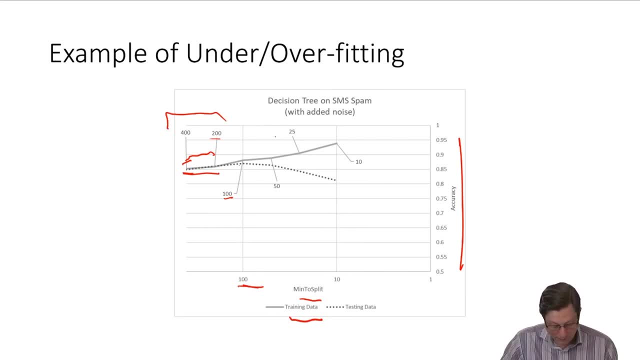 we've got a gigantic problem. when we move on to mint a split of 20 and to 10, you can see that the uh training set accuracy is going up, up, up, up, up. fantastic, just using the training data. you are on your way, you're in it to win it. this sms spam problem is going to be solved because of you. 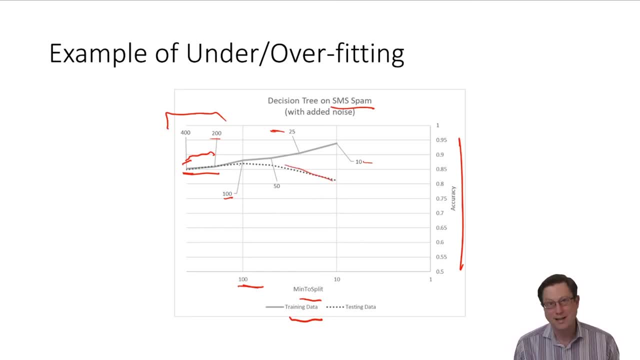 but then you test on the test data and things are getting like way, way, way, way, way, way, way worse and this is a very clear sign that your modeling process, with this particular value of the hyper parameter and whatever features you've chosen to use, however much you've exposed to the model, this is, this is starting to overfit you are having. 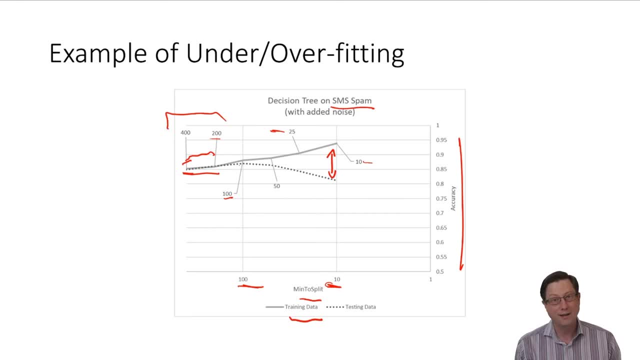 variance problems, you are overfitting the training data and you are not going to generalize. well, push it one more point and eventually, with a decision tree and really no constraint on how many splits a decision tree can put into the model, you're gonna get pretty darn close to 100 accuracy. 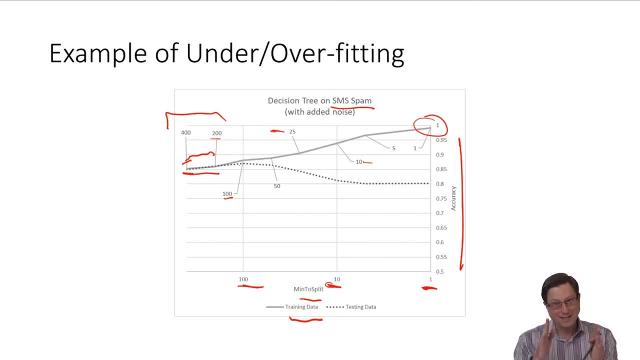 like really pretty darn. i mean there could be training examples that have all of the exact same features and randomization in the labels. so you, you may not get perfect, but you're gonna get very close to perfect, um, and then you'd see, in this case, that the uh generalization accuracy is 80 percent. 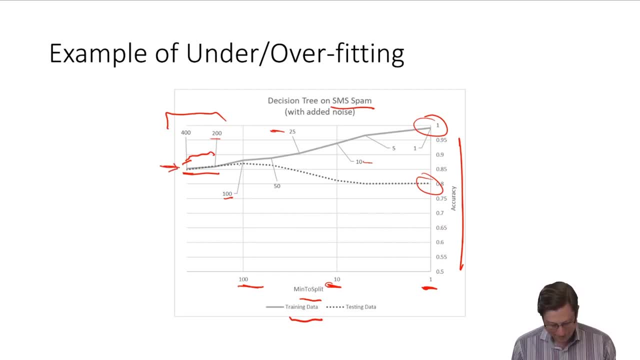 which was worse than when you had min to split of 400. so the the signal you're getting from the training data would clearly say to set this parameter to one. but when you're testing with the testing data, you're saying, well geez, i'm starting to overfit and in fact, the best value. 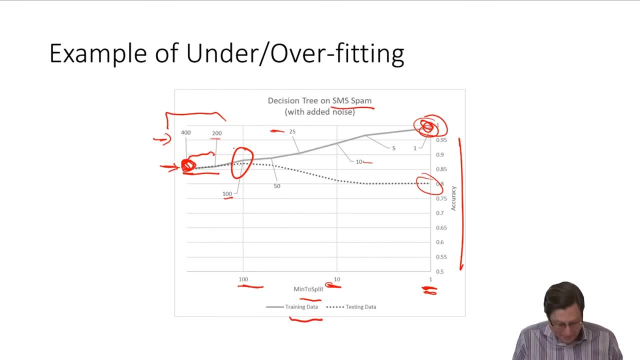 for you to use just by eyeballing this chart would be something more like a hundred. and that's the point where there is a little bit of a gap between these two, and that's fine. no, you don't need to have no gap. what you need to do when you're doing machine learning is produce the model that. 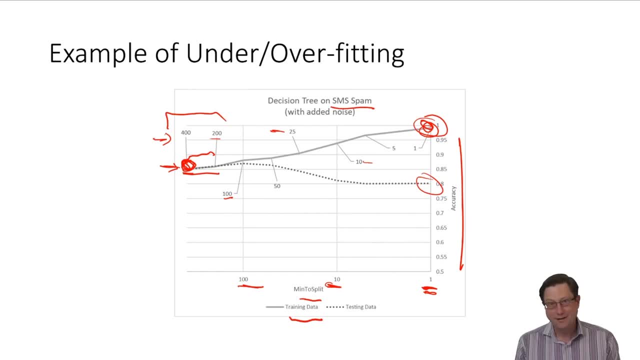 performs the best on the test data. not, you know, it doesn't. you don't need to produce a model that's not overfitting. you need to produce a model that trades off the problems you have with overfitting with the problems you have with underfitting. so you don't need to have a model that's not overfitting. 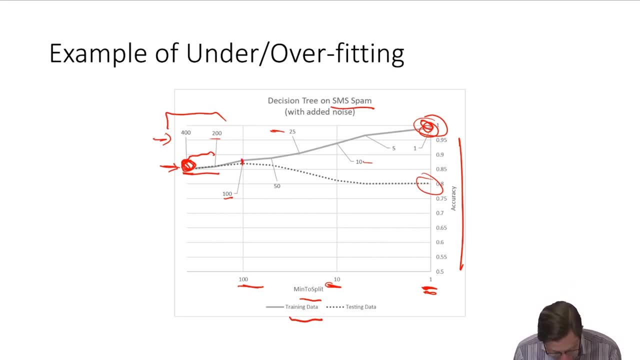 even though you'd say like, oh, that's not perfect in terms of the overfitting sense, it's the model you would want to use. you'd want to set this parameter to 100 and then start doing maybe sweeps on other parameters to see if you could somehow tease loose other sources of problems to. 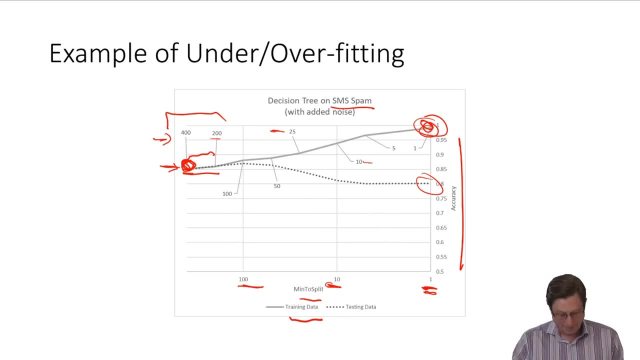 drive things even further or put another way. you know you've gotten. this is as far as you can get with this parameter. go come up with some other parameters, go come up with some other features, go try more things and you probably get further than this. so when we did the decision, 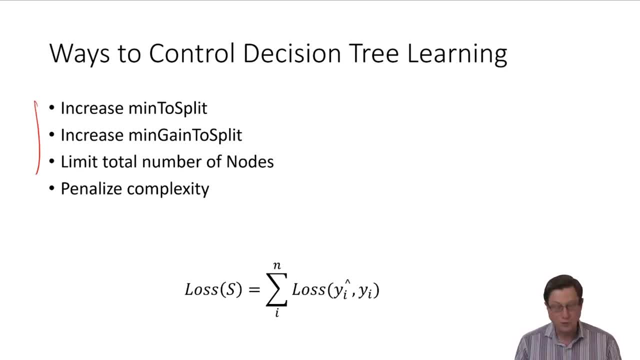 tree lecture we saw that there were all these different hyper parameters that you could choose to use um. and now you know why you might choose to use them and which direction you would point them in um. you know, i not going to go through like let's just say that it's empirical question. 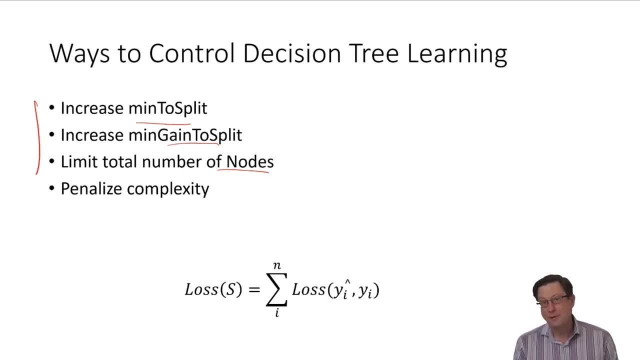 like: try the one you want, try multiple of them. do the parameter sweeps, like we just saw on that previous slide or maybe the slides. that way i don't know which way is behind and which way is ahead. um, but another way to think about it is that you could say: 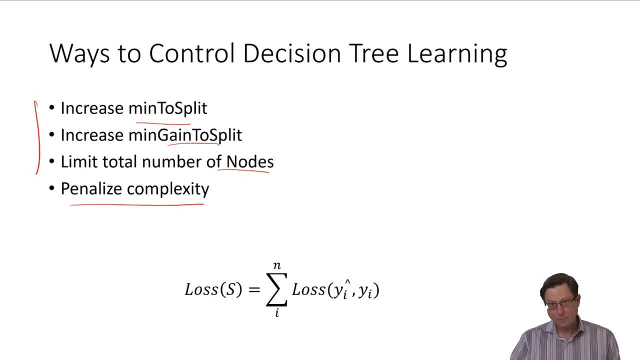 as i allow more structure into my model, i'm increasing the risk that i'm going to overfit, and so i'd like to add a penalty to the loss and this, might you know, i'd like to add my inductive bias into this loss, to say like: don't learn something too complicated, occam's razor remember. 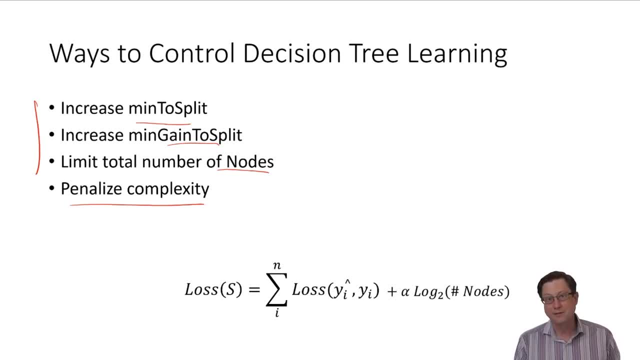 we talked about that, and one simple way you could do it is just add this parameter to the loss. and so then you would say, like i take the loss that my model has by um looking at how well does it predict the training data, and i add in alpha times some penalty for the number. 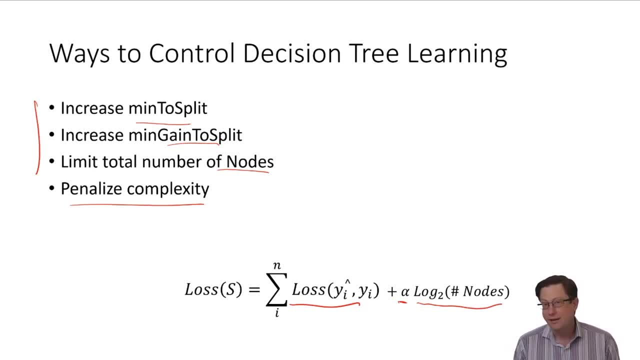 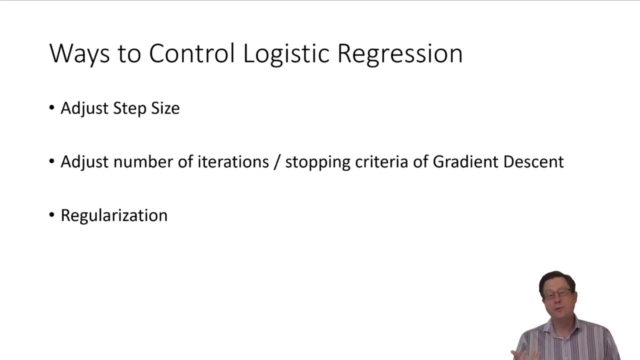 of nodes in the overall tree that i've learned, and then i pick the model that you know minimizes across this joint thing instead of just minimizing on this side alone. it's just another way to think of how you're injecting your inductive bias into the loss of this, and similarly we had hyperparameters for logistic regression. there weren't quite as many of them. they were: adjust the step size, control the number of and similarly, we had hyperparameters for logistic regression. there weren't quite as many of them. they were: adjust the step size, control the number of gains. and in order to make this stable analysis, we had to moderate Griffin on training data, data data for logistic regression, the mostrocket, best looked after and 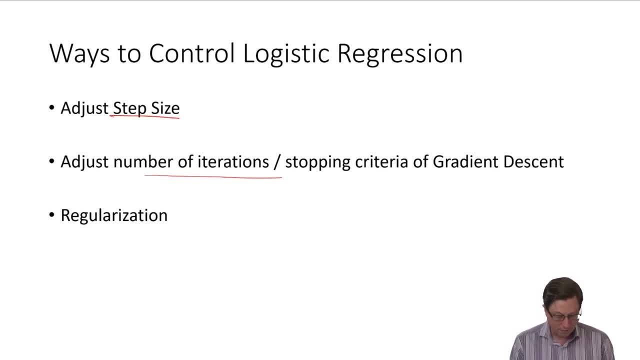 uh, they were, adjust the step size, control the number of of iterations or the stopping criteria, And we'll talk about regularization here in a second. But you know, by, by taking larger steps, you learn more concept more quickly. but you also are sort 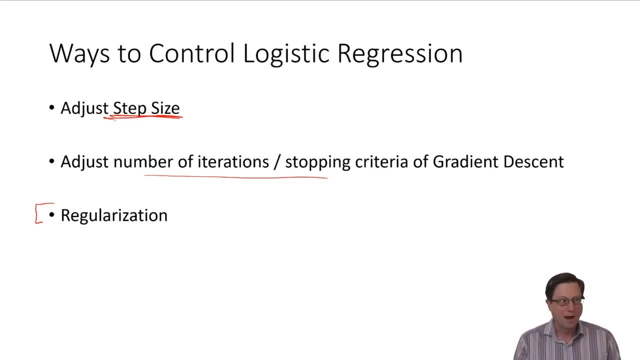 of quantizing the space, like you can't get all your parameters to exactly the same values, because you're you're taking gigantic steps versus taking very small steps. it might take you a long time to get there, But you really can wedge yourself down into the real bottom of the 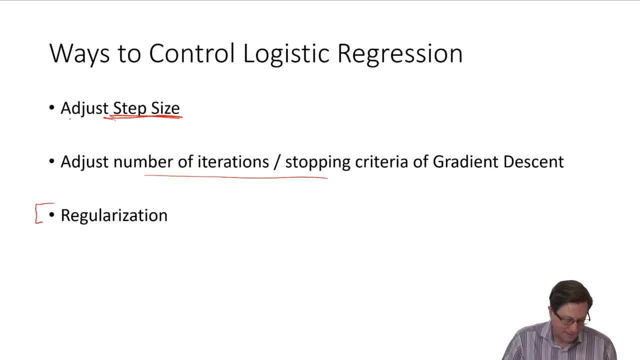 global optimum that you're going to find And and right, like adjusting step sizes for logistic regression. I mean there is a global optimum, So the step size determines sort of how close you can get to that roughly. in neural networks the space of your loss- surface space- is much more. 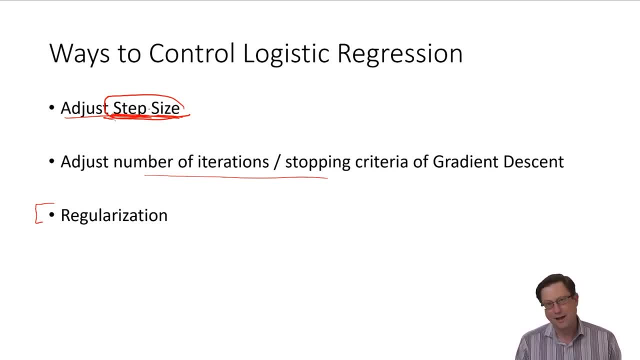 irregular, So adjusting the step size there can have a larger effect. we'll get there. Don't don't need to learn too far ahead. And of course, like you know, if you have fewer iterations or coarser stopping criteria you're not going to get as close to I mean, you just don't have as much. 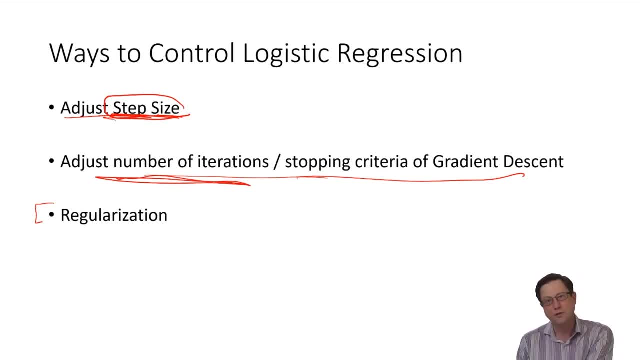 range to get away from the initial parameter values towards whatever that global optimum might be, assuming that global optimum might overfit. Another thing that people commonly do, which which we didn't do when we looked at logistic regression, is this thing called regularization, And it's 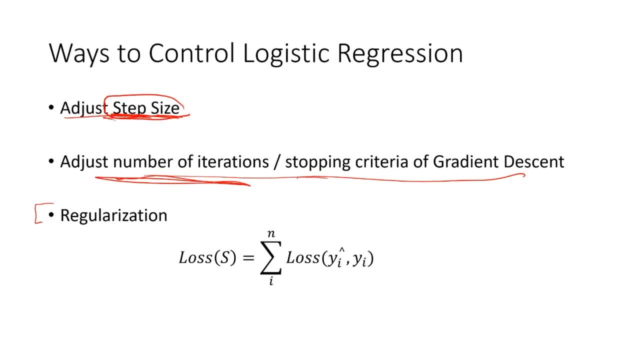 similar to what we did with decision trees, where you take the loss that you would like to talk about and then you add some extra cost. In that case you're not going to get as close as you would like to talk about. So in this version of regularization you'd say alpha times the sum of 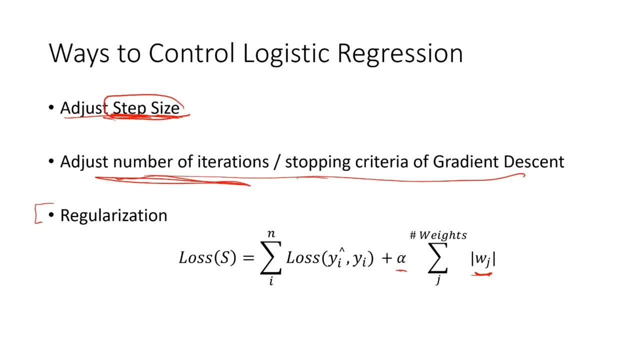 the weights that I have for all the parameters. So what does this mean? you start with weights equal to zero and then each step of gradient descent could add or subtract to the weights, And what this is saying is that you know, every time we take a step away from zero, that actually 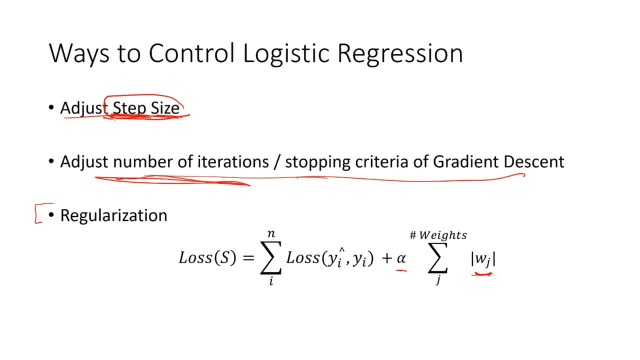 increases the loss, or I want to encode my inductive bias that those weights should be small. Now, with this set up for encoding that, it's called l one regularization, because it's the absolute value of the weights. In some sense this has built in feature selection because if you you think about this a little bit, 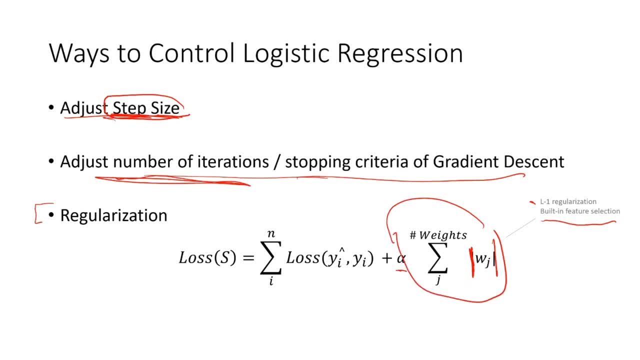 if there is a feature that is not helping you reduce your loss, this is going to set its weight to zero. you're going to absolutely prefer having a weight of zero for a feature that doesn't contribute. So after running logistic regression with built with l, one regularization you could. 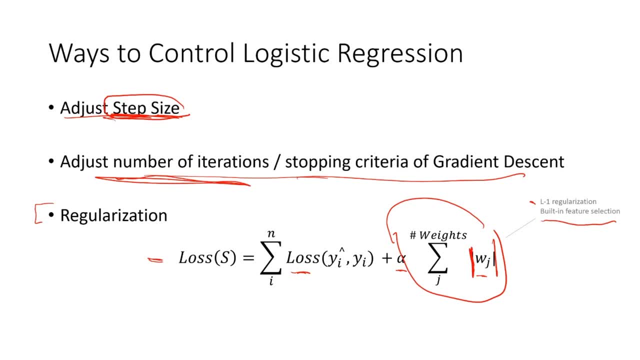 go and, you know, throw away every feature that has a zero weight, fine. Another thing that people often do is this version, where it's the weight squared and you know, square l one versus l two. this square would mean that you 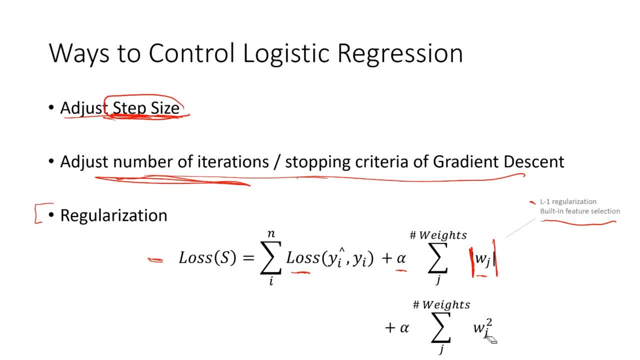 penalize large values more than you penalize small values. A couple of nice things to do about this is that you can take the derivative here, And so you can just fold this right into your gradient descent process, And that's what I mean by analytic solution. These would be, again, hyper parameters. 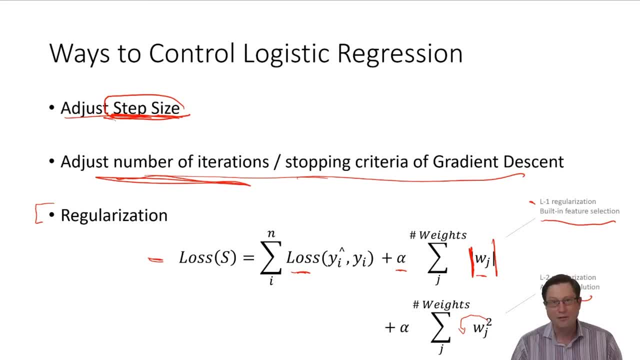 that you would try of turn on l one regularization with a particular alpha or l two regularization with a particular alpha, And that would be Another tool in your tool chest when you're trying to get the best tuning of a logistic regression model and trade off bias versus variants. All right, now you want. 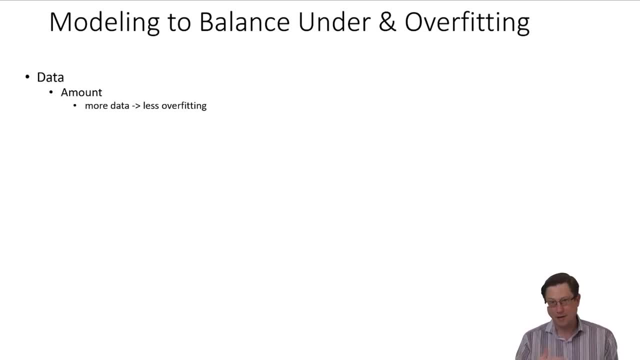 to look at even more tools in your tool chest that can allow you to make better bias variance trade offs or a better trade off between overfitting and underfitting, And you'd say that data Machine learning. people always want data. Give me all the data. I need all the data If 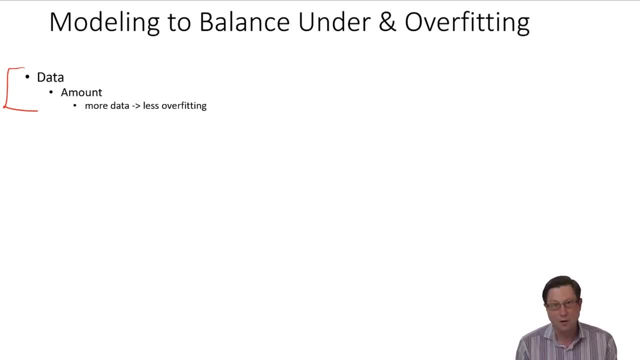 you're not giving me the data, it's because you want us to fail, and I don't know what's wrong with you. So the main reason is that more data leads to less overfitting, all things being equal, because it's less and less likely for your model to accidentally fit training data when you have. 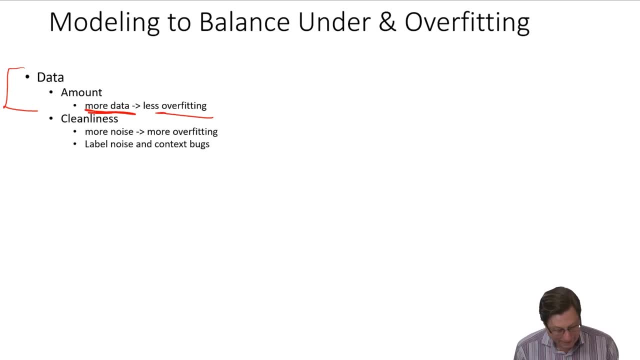 a heck of a lot of training data. The other thing you could do is clean the data. clean the data and you hear machine learning professionals. they joke around. you go on LinkedIn or whatever and see all these data scientists posting. It's like my job is 80% data cleaning. 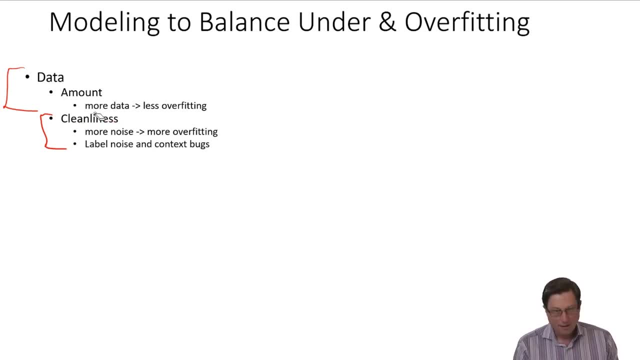 25% meetings and 5% modeling, Because when you have noise in your data that you could actually go and control, I mean you have to go control. You're shooting yourself in the foot. It's terrible. It's terrible. So you can spend a ton of time trying to figure out: is there noise in? 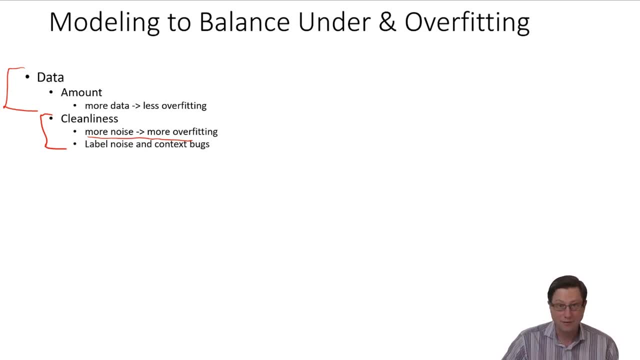 the data Because, if there is, it's going to lead to overfitting because you're going to get confused by that noise. The noise is going to happen to be correlated with the labels in your training data and you're going to happen to learn the wrong thing. 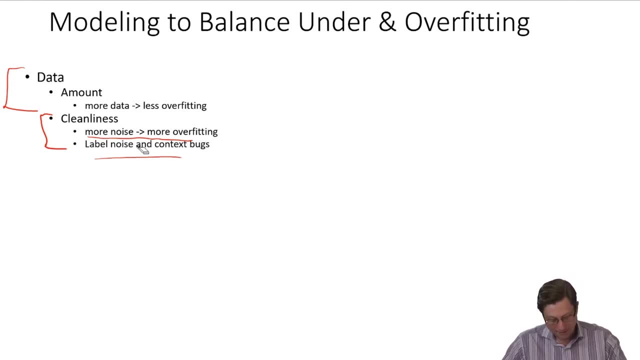 Label, noise and context bugs like errors in your logging. it's terrible. You're going to have to chase a lot of that stuff. if you're a professional machine learner Learning algorithms, you're going to find the algorithm that's best aligned with your concept, If you have a representation that. 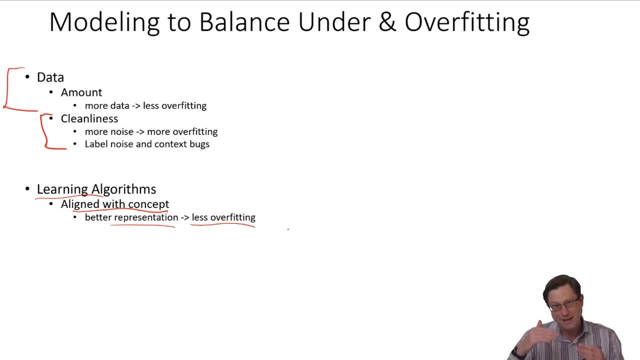 matches a true concept. you're going to have less overfitting because it's just easier for your model to slot in there. You can hit the contour between the different class labels without having to try to approximate it with a bunch of garbage And put another way. if you can hit the contour of the concept with less. 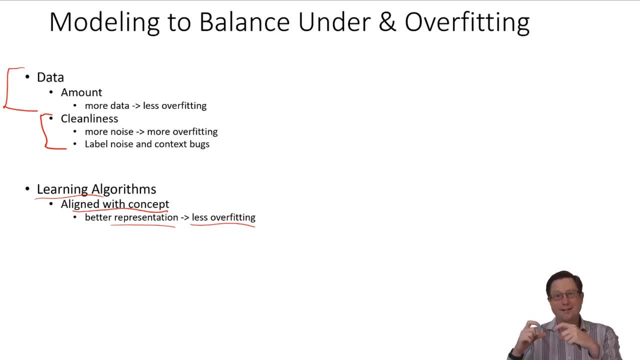 search because your model structure matches it. then you don't have to do more search and you don't have to push your model to try to piecewise approximate whatever the decision boundary happens to be. More power in your model leads to less bias, but more variance problems, And so as you go into 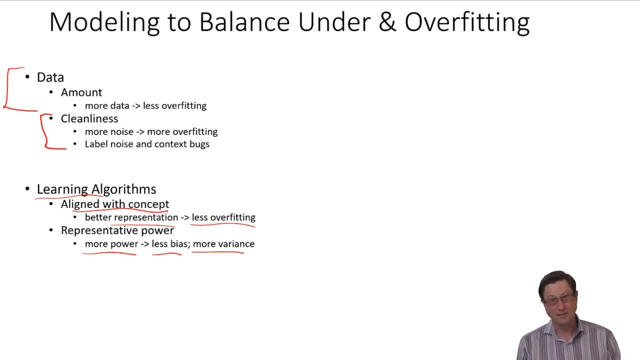 logistic regression. our parameter sweeps were pretty simple. There's not much to do, maybe some feature selection. As we get closer and closer to neural networks, you're going to have gigantic loops of trying things and trying to avoid, you know, getting the overfitting problems overwhelming. 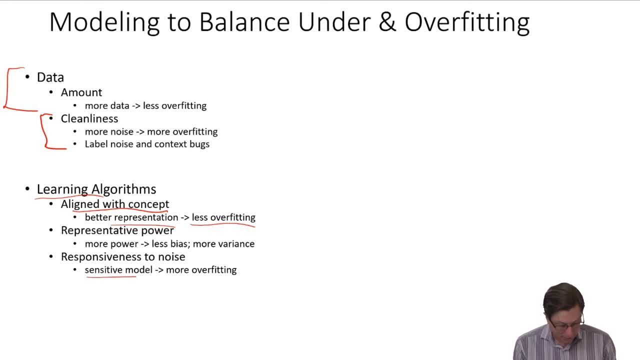 your ability to use your neural network. Some models are sensitive to noise and that'll lead to more overfitting, Like we saw. logistic regression can't be too sensitive, but decision trees can be Feature sets. feature engineering is very important because this is where you are. 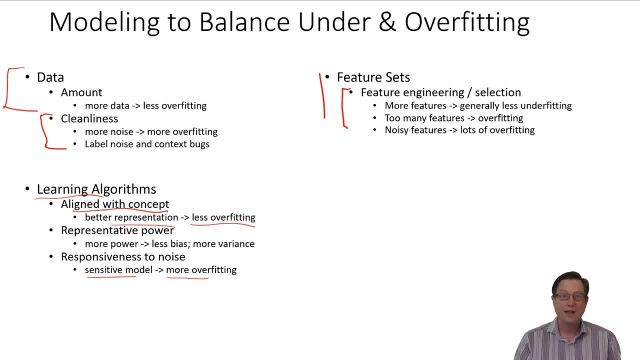 telling your model: hey, here's all the things to consider, And if you tell it some things to consider that aren't correlated, you're going to have it chase its tail, chasing these things that you've told it to consider that it really shouldn't. So, in general, if you do feature engineering and add more, 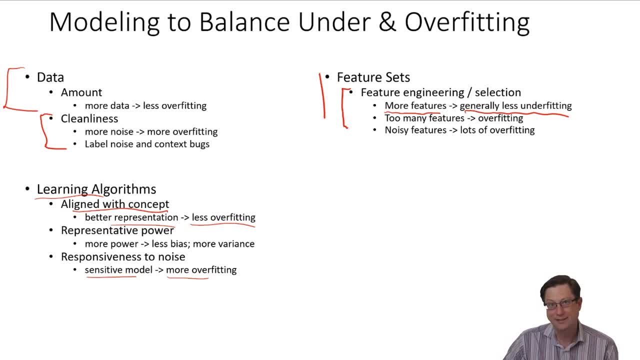 features, you're going to have lower bias, you're going to have less underfitting. But if you have too many features, you're going to have more overfitting, Because, no matter what, even if they're pretty darn good features, they just give you more ways for the learning algorithm to 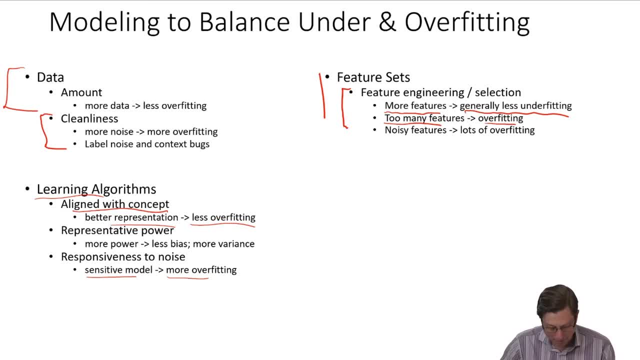 learn the concept the wrong way. It's just more opportunity for it, And particularly if there's noise in your data in any feature- and there always is- but you may want to think about it like, hey, this is a really noisy feature. I like it, but it's got a lot of noise I have to use. 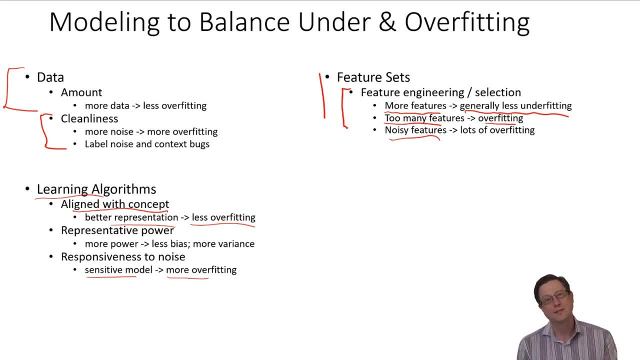 decision trees and I have to do a lot of search. Oh, I just can't use that feature because it's just going to distract decision trees. So this is a type of thought process that you might want to have: Search and computation: less search will generally lead to less overfitting and more. 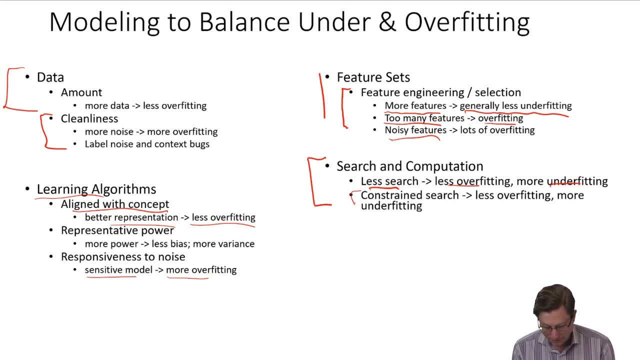 underfitting And constraining your search. conversely, you know you can flip it around, And so you'd want to control your optimization process. And then a great tool that you have. that we've just barely scratched the surface on. 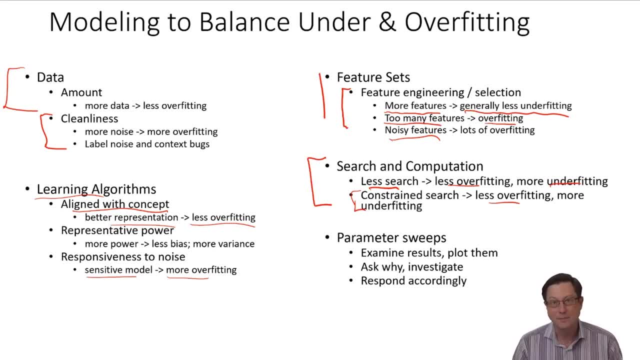 how to use the tool in this lecture And you're going to get more and more of this through the assignments And I think we'll have another lecture where I go into it in a lot more detail- But parameter sweeps are what allows you to figure out where you are in terms of overfitting and 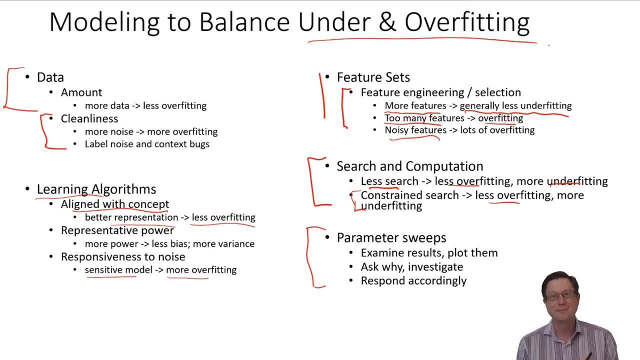 underfitting And hopefully because of this lecture you now have some sense of: oh, I look at this type of structure. I have an idea about what to change or how to direct my hyperparameter search And just a few notes on that is that: examine the results of the parameter sweeps Don't. 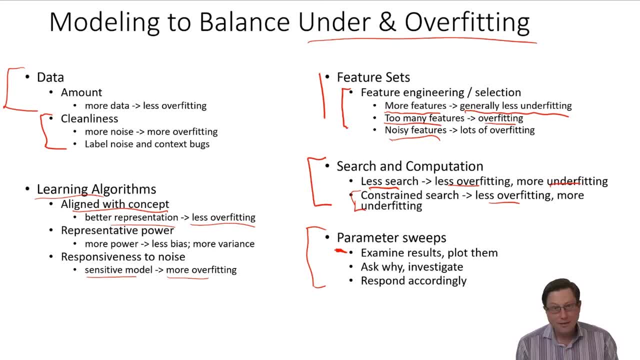 just try every possible parameter and be like, okay, this one had the highest accuracy, I'm going to ship it. Look at them, plot them in a couple of different ways and ask why? Why would that be happening? Why would that structure be looking that way? Why is it when I push that parameter? 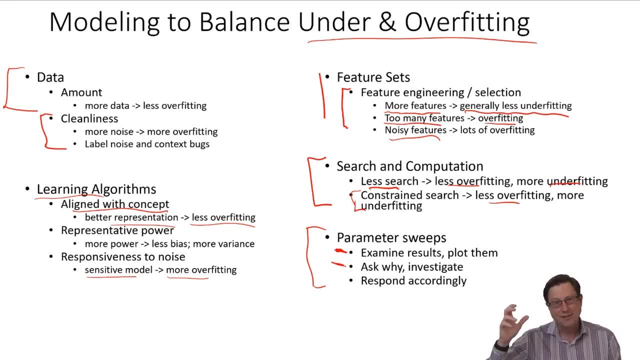 value higher, I start to see this change In the output, in the generalization accuracy. but when I push it lower I see this other change. And then, as you build up your intuition and your understanding of these fundamental concepts of machine learning, like bias and variance, overfitting and underfitting statistical bounds, 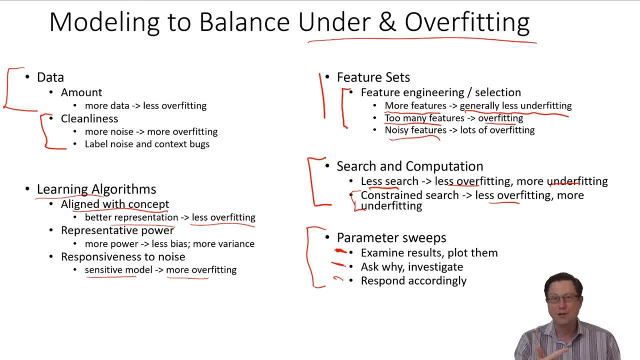 what is this data telling me? What are the knobs I have? What are those knobs do? That's when you're going to start to become an actually very good machine learning model builder. And a quick summary of what we covered in this lecture. 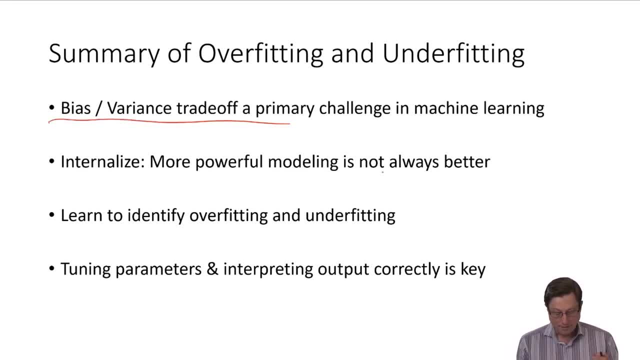 Bias and variance tradeoff is a primary challenge in machine learning. There's no way around it If you're doing professional machine learning and you're not thinking of bias and variance and you're not looking at every output and asking how bias and variance is affecting that output.